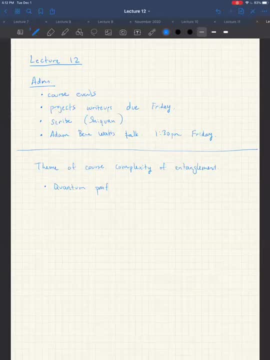 you know, comes up in a very natural way when we're thinking about problems from from any body physics, Like when you want to prove to someone that a a lot of the problems that you're thinking about are from you know, from any body physics. 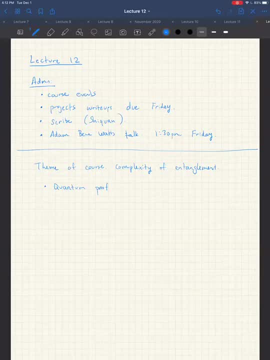 So, for example, if a local Hamiltonian has a low ground energy, the most natural thing to do is to just hand someone a supposed ground state that they can verify right And it's. and there where entanglement comes in is because these ground states can, in general, be highly. 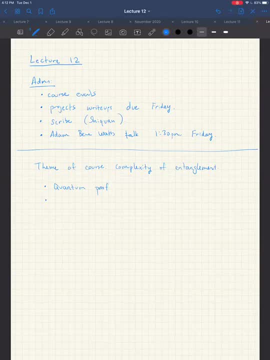 entangled. So you know you can't, you don't hope to that. there's a succinct, classical description of these states because they're highly entangled. So instead you provide them in quantum form and and that's, you know, very useful for efficient verification. 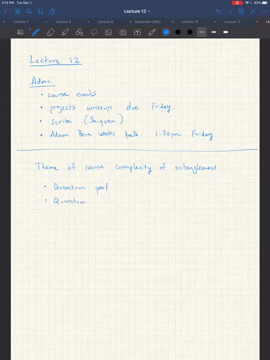 Along those lines. we also talked about this thing called the quantum PCP conjecture right, And this talks about how it posits the existence of these physical systems, these local Hamiltonians, where, even if you're, you're looking at the, the regime of relatively high energies. 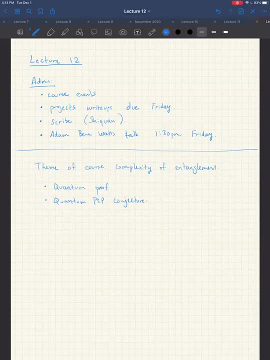 right, You know if you're looking at. you know if you're looking at. you know if you're looking at. you know not. you know not not things that are very, very close to the ground: energy. 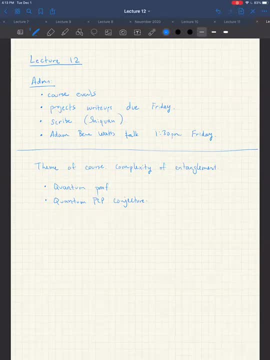 but? but somewhat far away from it. you still expect you know really complex entanglement to persist, right? Just to list a couple more things. we have verification of quantum computations, right? So here the the motivating problem is: you want to check that a quantum computer is really doing the. 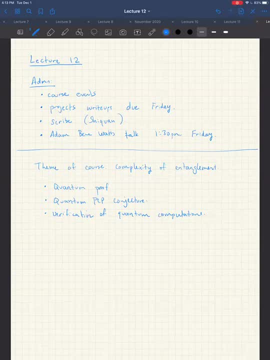 right calculation. You know how can you do this without having any quantum power yourself, And it turns out that by playing these non-local games with quantum provers as a classical verifier, you can certify that, first of all, these provers are sharing specific types of. 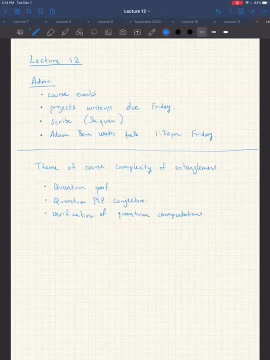 quantum entanglement. They're performing specific types of measurements And based on this, you can bootstrap yourself to verify full-fledged quantum computations. right, And so we saw a protocol. you know how to do that, And then you know. the most recent thing we talked about is 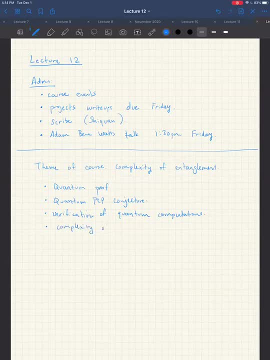 you know sort of thinking about the complexity of non-local games, right? So you have these games. these provers are allowed to choose some type of entangled strategy to try to win the game with as high a probability as possible. Can you estimate the winning? 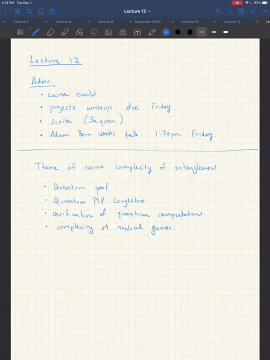 probability, And we saw that, in fact, there is no algorithm for this. So you know, so hopefully you see, like how this, this theme, really goes through all of these different topics. For today, though, we're going to talk about something seemingly 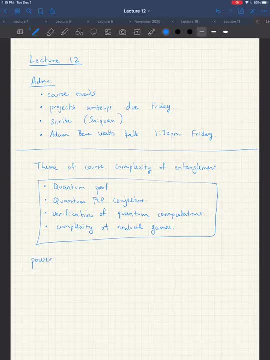 quite different. We're going to talk about the power of unentanglement, So we're going to talk about this in the context of a complexity class called QMA2.. All right, so, and we're going to talk about this in the context of a complexity class called QMA2.. 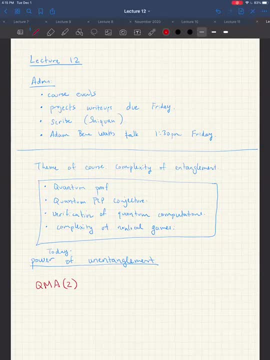 And you know, this is a model of quantum proofs where Merlin, the person who's creating the who's creating these proofs- is sending you not just one quantum state, but two quantum states, with a promise that these two states are not entangled. so maybe i'll write it this way: these are quantum proofs with an unentanglement guarantee. 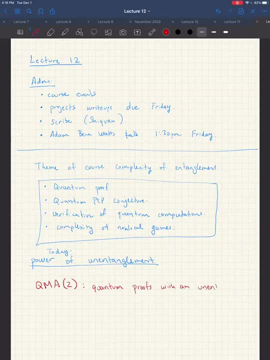 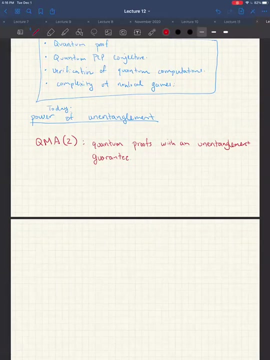 and um, to be honest, we don't know that much about this class. it's really mysterious, but it's one of these um, uh uh complexity classes that we'd really like to know more about. um, so so let me just- uh, you know, say precisely what is this model of unentangled proofs? 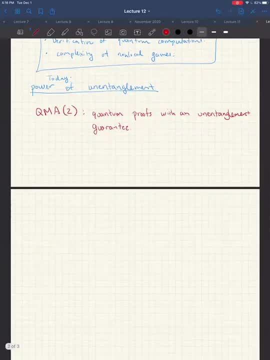 right. so just to uh remind everyone, um, let's recall the traditional qma style of proof verification. um so we have, um you know uh, a decision problem l and we want to know whether some instance is a yes instance or not right. so, for example, you know the local hamiltonians problem- we want to know if 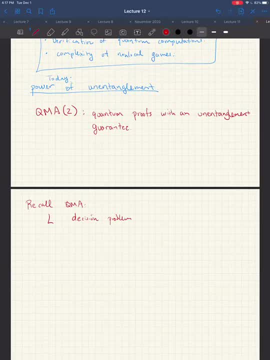 local, hamiltonian has a low ground energy. so, um, you know, we're given, instance, x, um and uh, you know so. so there's, there's going to be a polynomial time quantum verifier. let's give them a name: um, arthur, um, so there exists, uh, poly time. 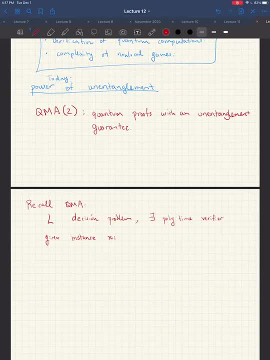 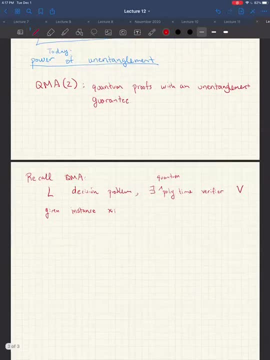 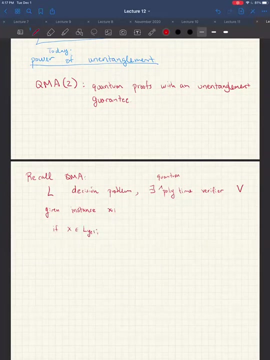 verifier v. okay, this is such that when it's given in instance x, if x is a yes instance, then merlin can concoct a quantum proof state. so there exists some witness state, psi, such that v, given the instance x and given the quantum proof, accepts with probability two-thirds. 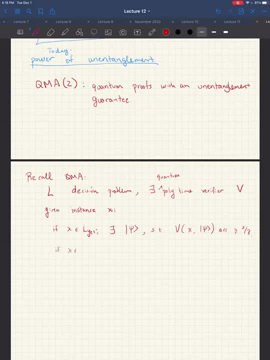 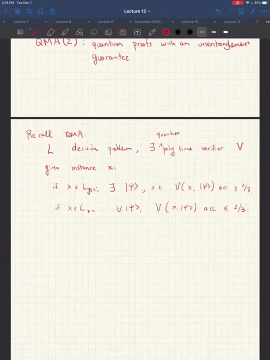 right. and then if, uh, if x is a no instance, then no matter what quantum proof merlin comes up with, arthur is going to not accept with high probability, so accepts the probability at most, uh, one-thirds right. so this is qma. uh should look familiar. um, now qma2 is is going to be very 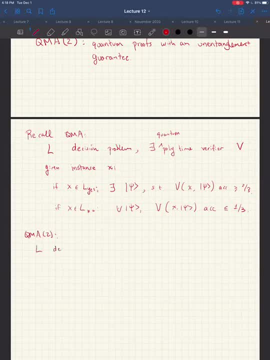 similar. um, we have a decision problem. okay, thank you. there's going to exist a? uh, quantum polynomial time. uh, verifier v. but the format of this verifier is going to look slightly different. um, it's going to have a. well, i will just sort of draw the the circuit. so here's our- uh, our verifier v. uh, it has a register that. 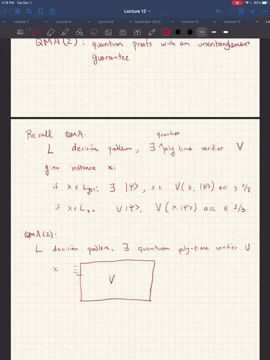 that takes in the, the instance x, okay, um, but it's going to have two verifiers that are going to be two proof registers. so it's going to have a, let's say, proof register one, p1, and proof register uh- p2, and it also has some um, a register for, you know, the, the n-cillars. 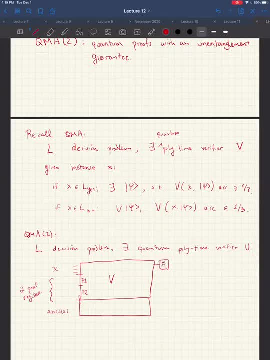 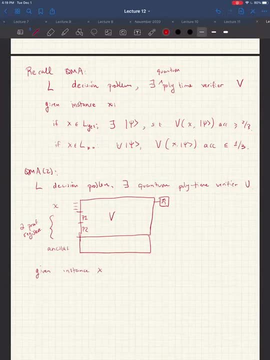 and then it has a you know accept or reject um bit at the very end. so, um given uh, instance x. if x is a yes instance, then there exists a quantum state, psi, on these two registers, p1 and p2, but it has a guarantee that it factors into this product state. 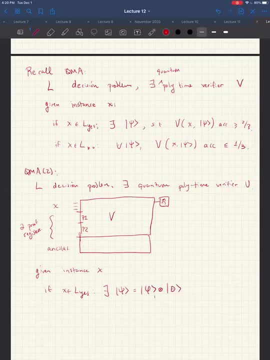 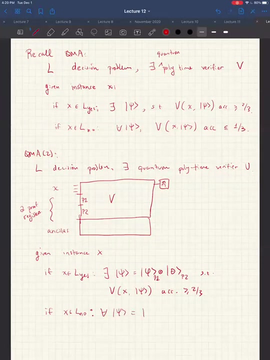 okay, so this, this lives in uh- p1, this lives in p2, uh, such that the verifier will will accept and in the no case we're going to say that for all states of this unentangled form, the verifier is going to accept, with probability at most, 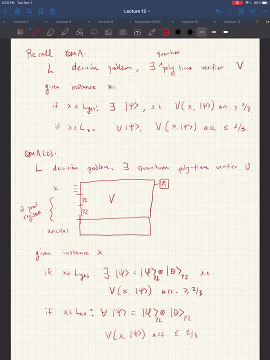 uh, one-thirds. okay, so everything is exactly the same. so we're going to say that for all states of this unentangled form. it's just that when we're talking about the proofs now, we we have it split right in the middle and the state is unentangled across that cut. so, if we visualize it, we have this psi here. 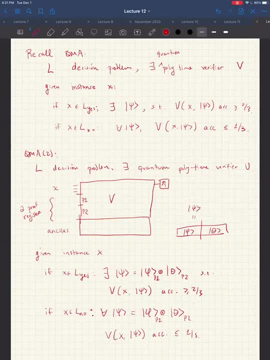 it must look like this: phi, tensor, theta. within each block, though, these states can be arbitrarily entangled, it's just across this cut. there's no entanglement between the two. so the first thing i want to emphasize is that, given this verifier, the first thing i want to emphasize is that, given this verifier, 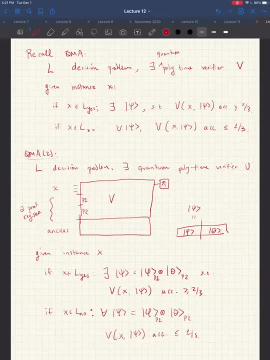 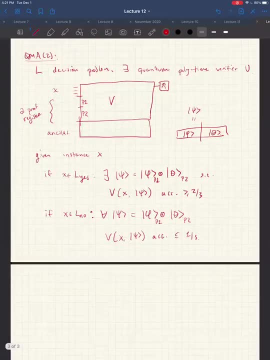 in both the yes and the no cases of this and the Pareto Isolation. i do want to emphasize that, even if we want to apply this into the, we want to be right on the same same place, so everything is going to be right on the same spot. 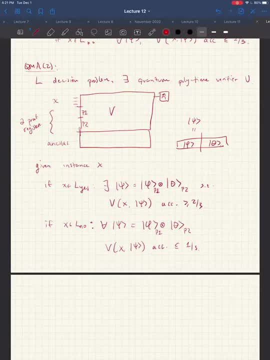 and the point is that, even though this was a very interesting one and it's been a little bit hard to get to, um, i've been very Ну, okay, um the yes and no cases. there is this unentanglement guarantee on the proof state, But we cannot say: 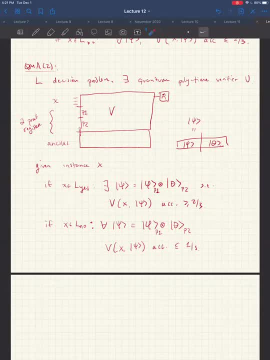 anything about what would happen if the state that was provided by Merlin was entangled across this cut? So, in particular, it could be that this x is a no instance, but if Merlin came up, you know, handed this verifier a completely entangled state that doesn't satisfy this unentanglement guarantee. 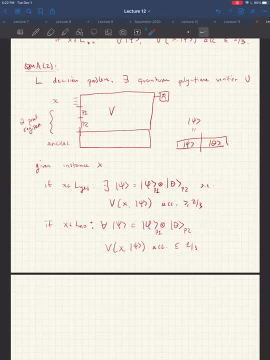 the verifier could get confused and accept when it's not supposed to. We only know what happens. you know the verifier is only clear on whether it's a yes or no instance. if there's this unentanglement guarantee, So that'll be quite important. 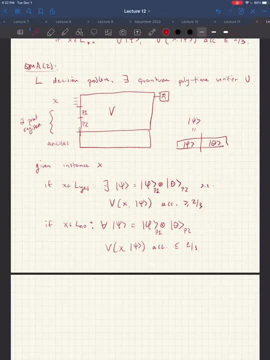 So we've, you know you, can you define this, this seemingly weird variant? but there's a natural question of: well, how does this compare to the original QMA that we know and love? right, It's a complexity, class it. you know there are decision problems that are verifiable in this. 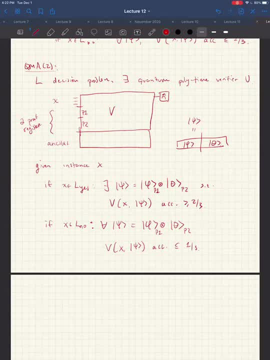 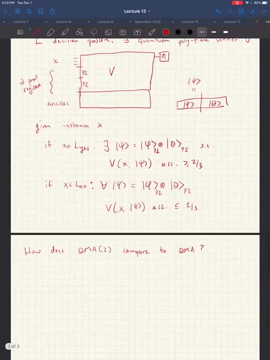 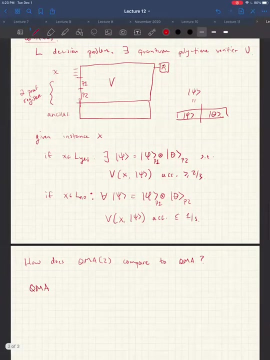 model. Can you verify more things or fewer things? So you know how? does you know? QMA2 compare to QMA. So the first thing I claim is that it doesn't. you know, having this unentanglement guarantee cannot reduce the types of problems that you can verify. 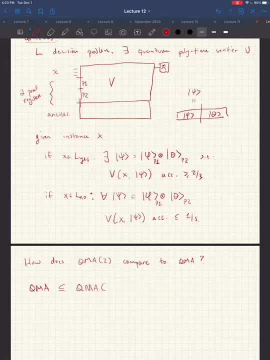 So in other words, QMA is contained in QMA2.. So does someone see why that this follows? You can always just use one of the two proofs. Yeah, exactly If you had a QMA style verification that automatically upgrades to a QMA2 verification protocol where you just always ignore this second register P2,. 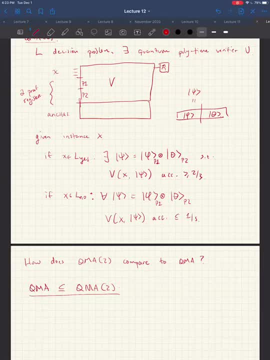 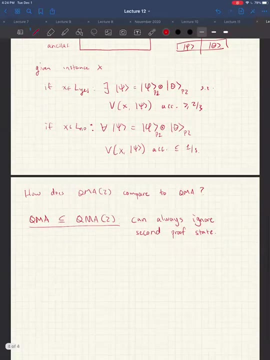 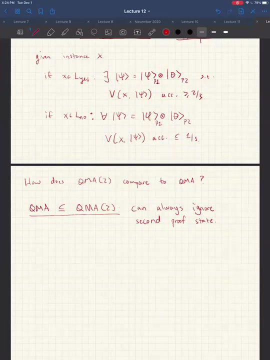 right. So you don't really care if there's this unentanglement guarantee, So you can always ignore the second proof state: Okay, so that's the easy direction And it's the other direction that's much more mysterious. In fact, we don't know, it's true. So you know this is the big open question. 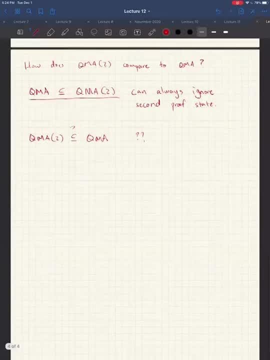 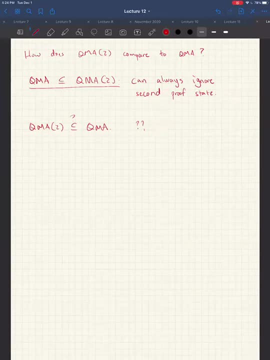 And maybe we can dwell a little bit on why it's not obvious that the reverse inclusion holds right. So you can ask: you know, why can't this normal QMA verification simulate the QMA2 verification model right, Like you know, why can't Arthur's? 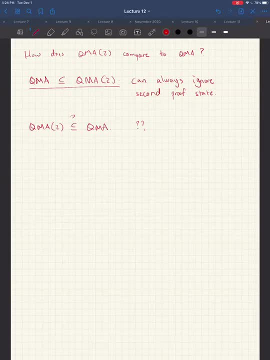 manufacture this unentanglement guarantee for himself. Okay, No, Arthur is the verifier. Arthur, You know, suppose, like you know, Merlin comes down and sends some arbitrary entangled quantum state, right? Yeah, Yeah, Yeah, Right. 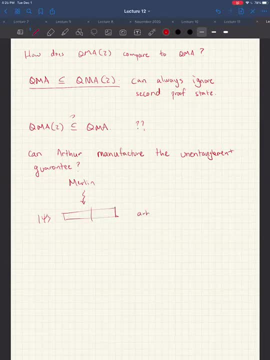 So it's not necessarily unentangled across the cut, So it's arbitrarily entangled across P1 and P2, right? Can Arthur somehow do something to, like you know, break the entanglement, so to speak, between between, you know, P1 and P2?? 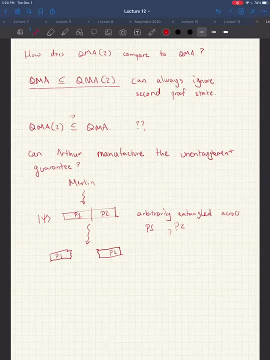 Yeah, p2.. So that's one thing you might hope is possible. Maybe I'm not following, but why does he need to break it? Why can't he be like? this is probably stupid, but like I got the state phi, I'm just gonna say okay. 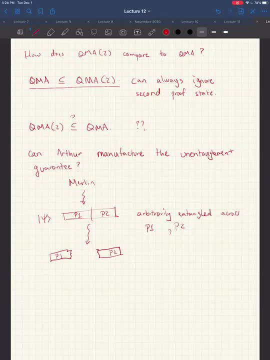 I'm gonna run the circuit on phi times phi or like phi times some dummy state, And that's a state that I could have gotten in the QMA2 protocol. So I should be fine on that, but I guess I'm not for some reason. 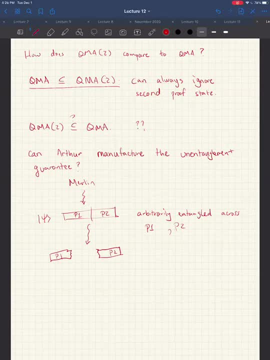 Let's see. so you wanna take, so you get psi, and then you wanna do psi tensor or something else. Yeah, and on this I'm going to run the ser, the ser, the circuit of the QMA2 problem that you gave me. 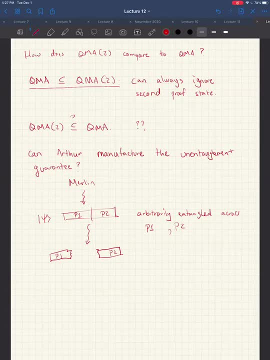 Sure, oh, you can certainly do that, but then you're you don't, but then you only have half of the. you only have one of the two proof states. What do you put in the second register? Like what? whatever, I want right. 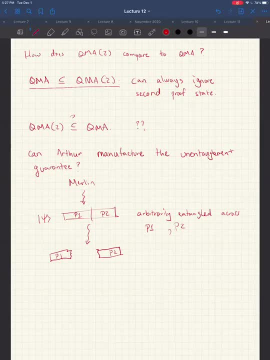 I know that for all proofs that look like a state, I'm going to accept the probability at most 1 third. So here you go, You have a proof which is a state times a state. Oh sure, Oh. so that's fine for the soundness, for the no case. 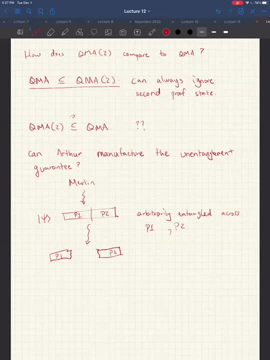 but what about the yes case? Well, isn't the yes oh, because they're supposed to be okay. okay, sure, sure, Yeah, yeah, okay, So you can deal with that issue, that issue. but then there's a problem that pops up somewhere else. yeah, okay, okay, yeah, good question. 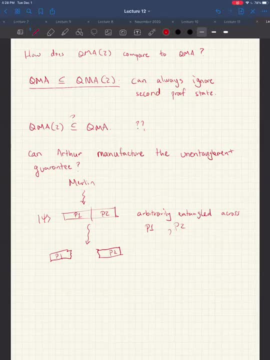 um, so you know, you can try to think of ways where arthur can try to like, force himself, force the situation to look like the qma2 setting right. so one way is: well, can i take a quantum state and sort of break it in half, like break the entanglement between the? you know? 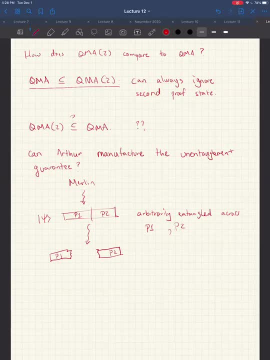 the left and right half, um, the. the basic answer is that, um, you know not, not in the way i described it. so you know that this is um, you know not, not really. there's no quantum operation that you can do. where you can, you know you get a state, uh, a psi, and then you can do some operation where you get. 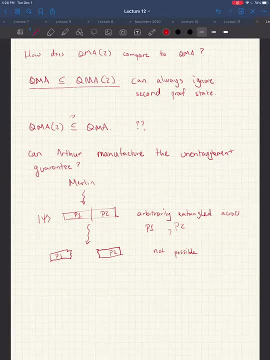 you know, um row one, tensor row two, where row one and row two are related to psi and and in in in the natural way, Like, for example, row one looks like the partial trace of psi on the first register and so on, right, So you know this kind of entanglement breaking. 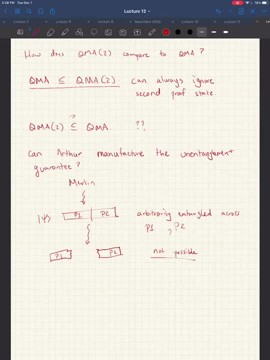 is not really possible. Another thing you might try to do is: well, maybe I don't wanna just break the entanglement, but can I at least detect whether there was entanglement between P1 and P2, right, If I could detect it and say, well, aha, Merlin. 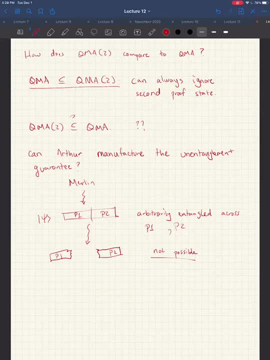 you're messing with me. you're sending me an entangled state I'm just gonna reject That would be great if it was possible, but it's also not possible in the, at least directly. So. can Arthur detect whether psi is entangled? 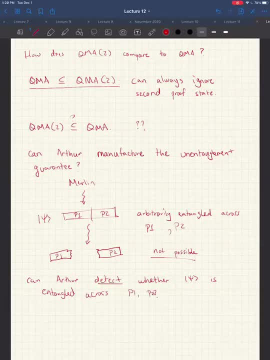 across P1, P2? And the the answer is: this is not possible. Right, Like what I mean by detect, is you know you can imagine maybe I can perform some kind of measurement on P1 and P2 that would accept all product states. 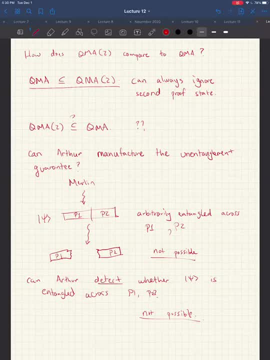 but reject all entangled states or something like that. And you know, you can quickly convince yourself- well, if you think about it for a bit- that this shouldn't be possible, because you know the set of states that span the, you can find a basis for the space of P1 and P2. 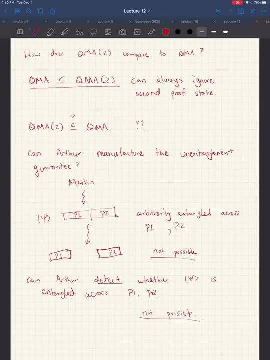 in terms of product states, right. So if your measurement accepts all product states, in particular it will accept all possible quantum states in the space of P1 and P2.. So it cannot distinguish between product versus entangled. So there's no measurement to distinguish. 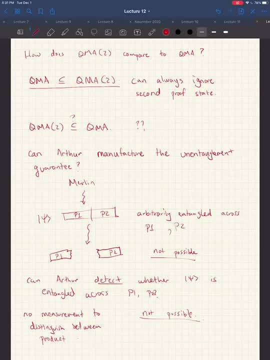 between product and entangled states. All right, so just running through this thought exercise, you know it's not so obvious how we can obtain this unentanglement guarantee, And so, in fact, this indicates that this guarantee is pretty special. 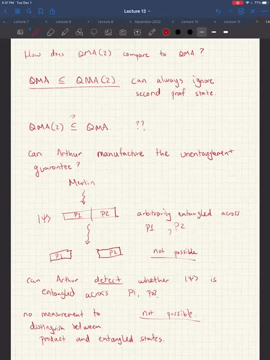 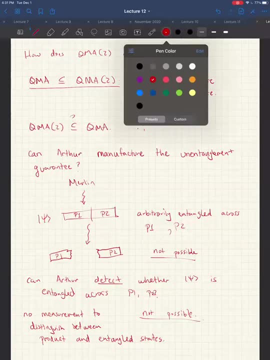 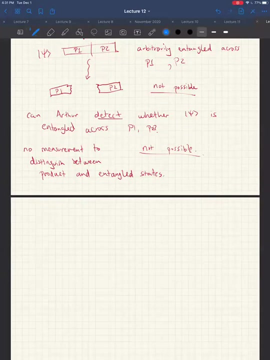 And so let's actually see an example of where you can do something with this unentanglement guarantee that you couldn't do otherwise, And so the application that we're going to see is we're going to see a a way of verifying NP right. 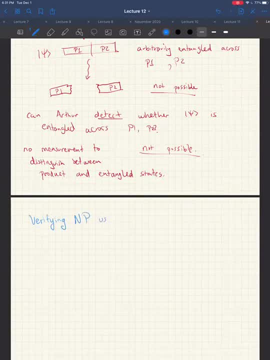 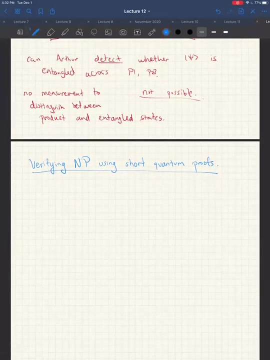 The. you know this classical NP using short quantum proofs. So we'll see how we can verify any NP decision problem using very, very succinct quantum proofs in the QMA2 model. So let's take a canonical NP complete problem. In this case I'll look at three coloring. 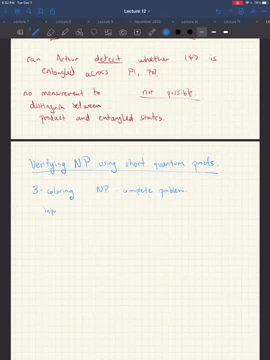 So what's this problem? You're given as input a graph and you know you need to decide. is there a way of assigning one of three colors to each of the vertices, such that when you look across the edges, the vertices have different colors? 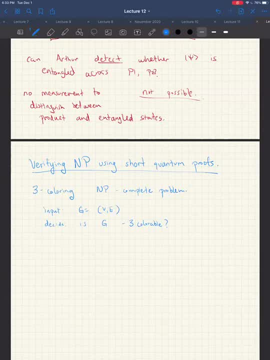 Is G3 colorable Right, And you know clearly this is in NP, because if you wanted to convince someone that a graph was three colorable, you would just give them the assignment to each of the vertices. like you know, this vertex is red. 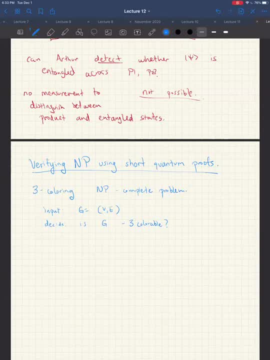 that vertex is blue, and so on. So so, three coloring is is an NP. And what is the size of the proof that you would have to give to someone to convince them of this fact? Well, if you had an N vertex graph. 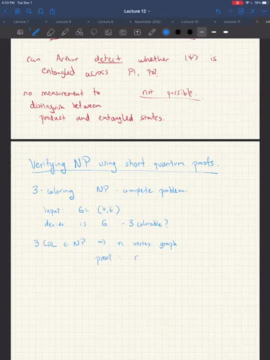 the proof, which is just a coloring, right, It's a coloring from the set of vertices, to say a red, green, blue. you know how many, you know how? how big is this proof? Well, you just have one color per per vertex. 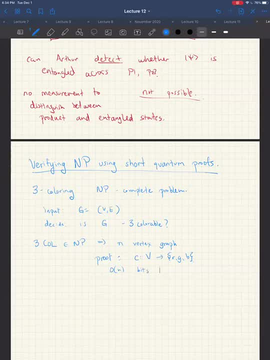 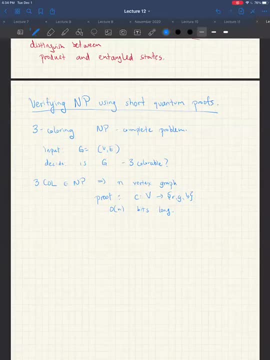 So so this proof is O of N bits long, Right? So that's kind of the straightforward way of writing down a proof for three colorability. So the question is: would it be possible to provide a shorter proof of three colorability? 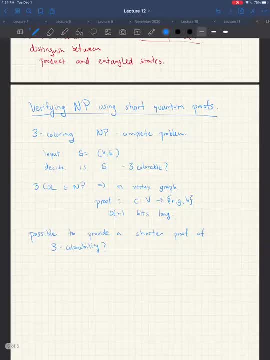 Like maybe there's a, you know, there's a more clever way of like compressing down the information in in a, in a coloring of a graph, right, Like surprisingly systemically it seems to be complex, But yeah, that really is the answer in my opinion. 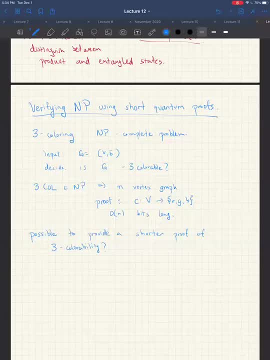 It is. So we had 10 proving proof of three colorability, a graph where if you have an N vertex graph, maybe the proof only has to be N to the 0.99 bits long. Right, that'd be kind of cool, because then maybe 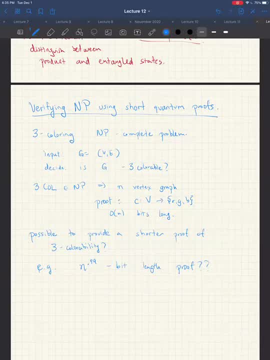 for some structural reason or some properties of this problem. you don't have to provide all of the colors, Any sense for whether this could be possible or not By intuition. if you know that one node is a certain color, you know that its neighbors cannot be that color. 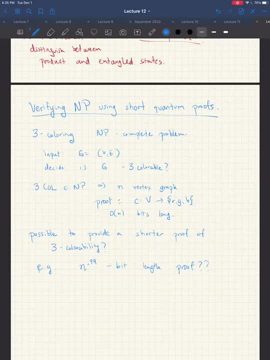 So I think that, like by intuition, it's possible. Oh yeah, That's a good point. So definitely there are certain shortcuts you could take. So, using that idea, you can sort of leave off one out of every three vertices or something like that. 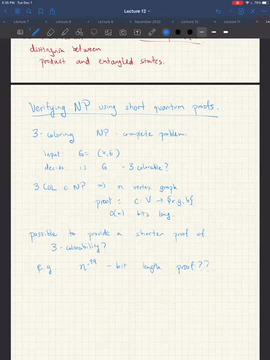 Oh, but that's still N over three. Yeah, I mean, there's some savings, So definitely you don't need N. but here I'm interested in something where you get like an asymptotic, something that's asymptotically smaller than a linear size proof like, let's say, square root N. 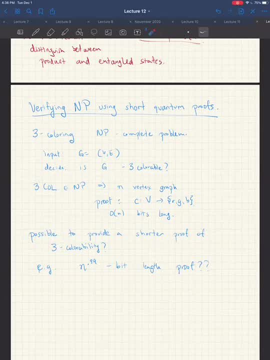 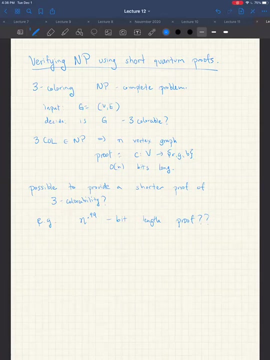 or something. Maybe you can hope that there are more observations like the one you just came up with. to come up with such a compression? Any sense on what does your intuition say? for that? I got nothing, Yeah, so to date we don't know of any such shorter proof. 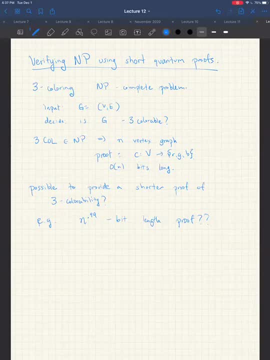 for three coloring And actually, if there was, this would actually have some like algorithmic implications. Suppose there was like a way of proving three coloring to someone. Yeah, You know, there was a proof system for let's say yeah. 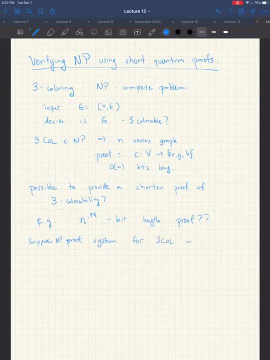 NP proof system for three coloring with M bit proofs. That would actually imply there exists in a deterministic classical algorithm a way to solve three coloring in time. three to the M, Sorry, no two to the M, right, And why is that the case? 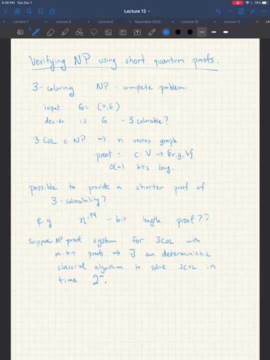 Well, this algorithm would just simply enumerate over all possible M bit strings, M bit proofs, and just check: does the verifier accept any one of them? If the verifier accepts at least one of them, then by the definition of the verifier you know that the graph must have been three colorable. 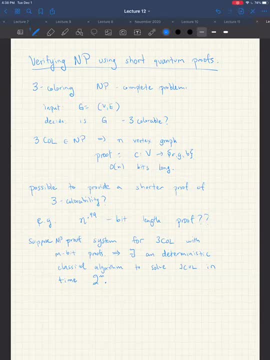 Otherwise it wasn't. So if, in particular, M was N to the 0.99, then we get a two to the N to the 0.99 time algorithm for, you know, for three coloring, And we do not know of such a thing. 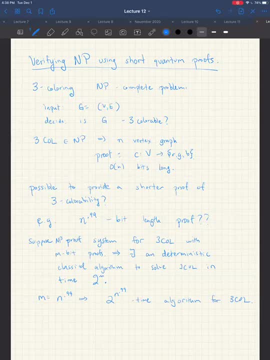 So this is a huge number, right? This is like some kind of exponential time, But it's not strictly exponential time. It's not two to the N or two to the constant times. N, Right, In fact, the best algorithms we know for many: NP-complete. 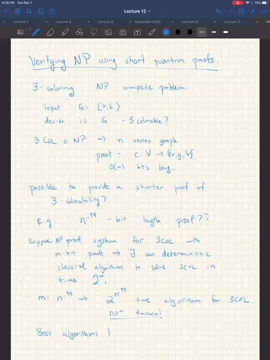 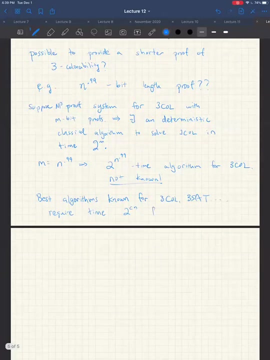 problems. You know, for three coloring, three set, you know you name it all take time. that's what's called strictly exponential. So it's some time, two to the C, times N for some constant C, And so we call this. you know this is called strictly exponential. 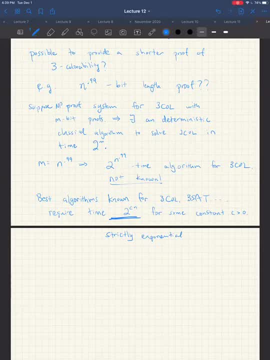 Anything that does better than this we'll call sub-exponential. So this is an example of a sub-exponential running time, And you know, this fact, or this strictly exponential runtime for these NP-complete problems is so pervasive that it's led people to formulate a conjecture. 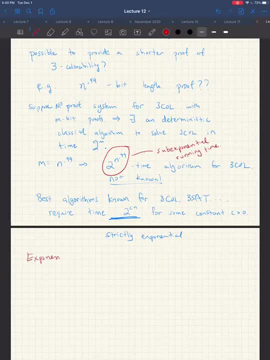 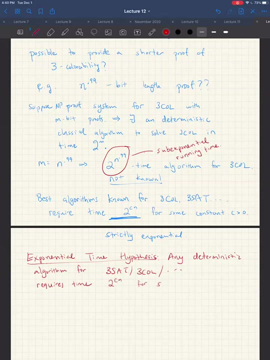 which is called the exponential time hypothesis Right, And it says that any deterministic algorithm for three set or three set right, Three coloring or you know many other natural NP-complete problems, requires time at least two to the CN for some constant C in the worst case. 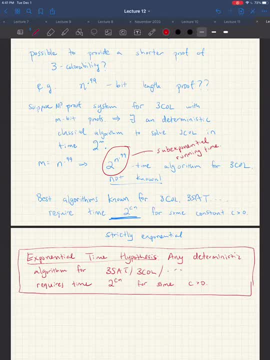 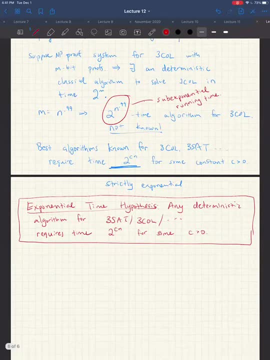 Right And all the evidence is, you could say, is in support of it. At least, we haven't found any counter examples to it, And this is a strengthening, Of course. if this were true, this would imply P is not equal to NP. 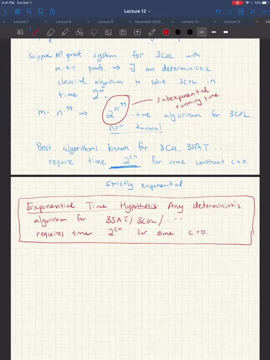 So it's, you know, should be hard to prove. So this is a strengthening of P versus NP, Right? We call this, you know, we give the shorthand- we call it ETH exponential time hypothesis. So ETH is the exponential time hypothesis. 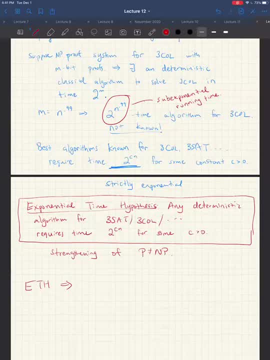 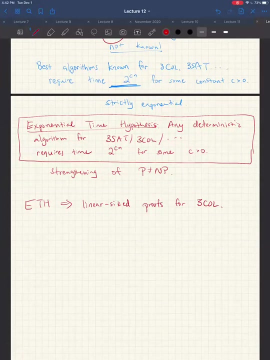 And ETH implies. you know, given this chain of reasoning, that we don't expect shorter proofs for three coloring, So we expected linear sized proofs for three coloring. Right In particular, you cannot hope to compress the proofs too much, smaller than some constant times n. 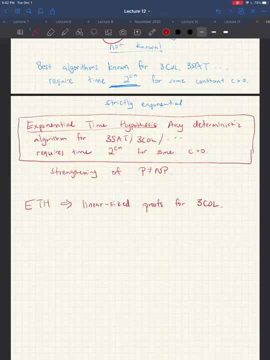 Any questions about this so far? So this is all classical stuff, right, So you know. but what about quantum proofs? What about the quantum world? Could we hope to do something better? Right, Maybe you know. let's say that Arthur wants to verify. 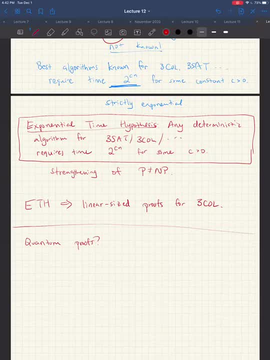 whether a graph is three colorable, and he's willing to accept quantum proofs to check this. So could Merlin send him a state of on n to the 0.99 number of qubits to convince Arthur of a graph's three colorability? 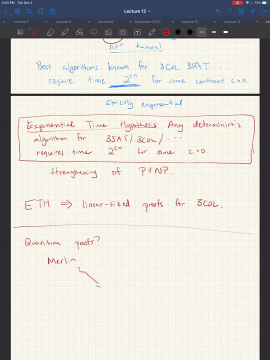 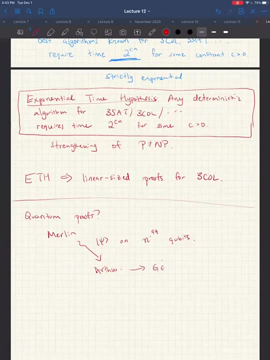 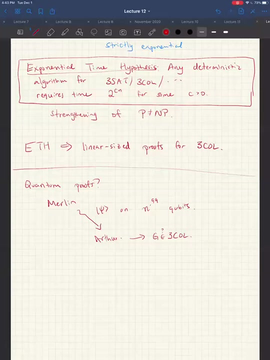 You know. so maybe Merlin could send a state to determine whether a graph is three colorable or not. You know, you can hope for such a thing, But again, the exponential time hypothesis implies that this shouldn't be possible. So, even though you allow yourself, 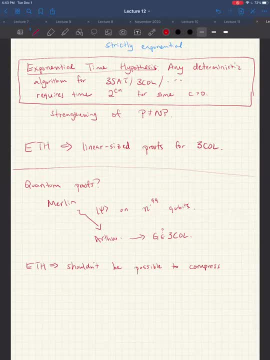 to store information in quantum form and allow Arthur to perform quantum computations. for this three coloring problem you shouldn't be able to have more succinct proofs. Is this obvious to see? Because you can't just say like brute force over all proofs. 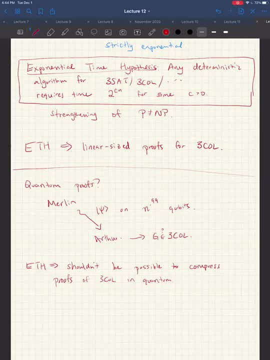 Yeah, it's not the same argument as before, because now the space of proofs is much bigger, in some sense Right Like, because if you have m qubits right, you can't just say like brute force over all proofs. 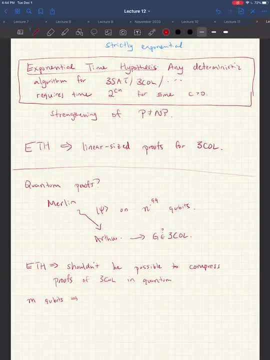 Right, Yeah, I mean, first of all, the space of all m qubit states is infinite. right, It's continuous. But even if you discretize, there's still a doubly exponential number of different proofs. Right, So, like, roughly speaking, there's a, you know. 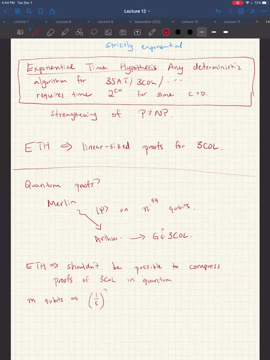 if you discretize to accuracy, epsilon, then there's 1 over epsilon to the 2 to the m. you know different quantum proofs to consider. So that's a, You know, which is way too large. But you know the argument goes as follows: 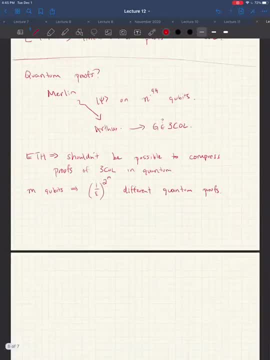 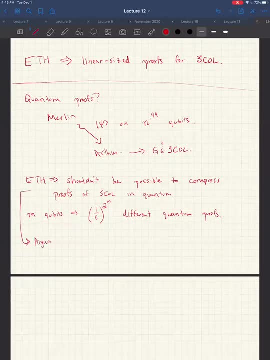 You know if you have a QMA verifier right for this three coloring problem. so here's the argument. So a QMA verifier for three coloring. so let's say that it takes an m qubit. It takes an m qubit as its quantum proof state. then let's: 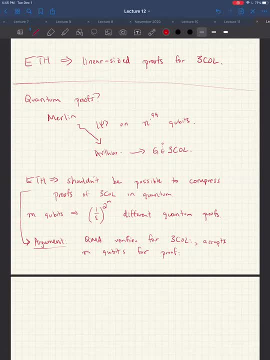 say you're a classical algorithm and you wanted to know whether the verifier would accept on some quantum state, then this is actually a maximum eigenvalue. problem Right. This is related to this thing you did in problem set one or problem set two Right. 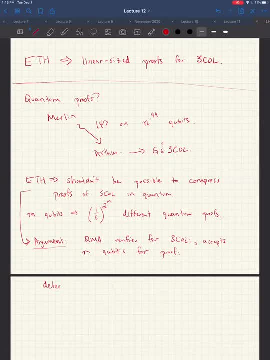 This is related to this thing you did in problem set two. So determining whether verifier accepts on some quantum proof is a maximum eigenvalue problem for a matrix that's of size two to the m by two to the m And this matrix comes from you know. basically writing out the description of this verifier: 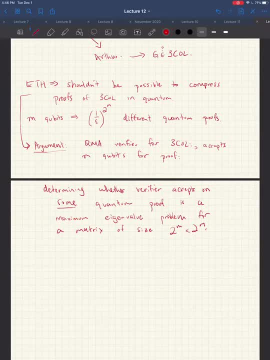 as like a unitary, and then you put in like the measurement that measures whether it accepts it or not, and so forth. Anyways, if you write it in the right way, you'll see that really you're just trying to maximize the maximum eigenvalue problem. 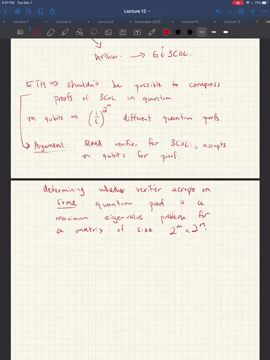 Right. You can find the maximum in polynomial time in the dimension of this operator, which is two to the m. So this is solvable in poly two to the m, which is equal to two to the some constant times, m time. So even in the quantum case, in this QMA setting, 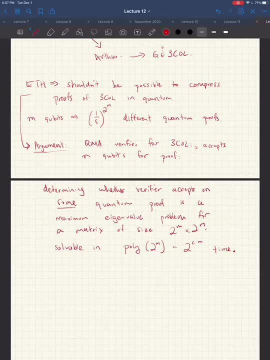 Right, If you could have n to the 0.99 qubit size proofs, then you would have a sub-exponential time algorithm for three coloring, which, according to ETH, we don't think is possible. So it seems like okay. well then, you know, maybe the conversation just stops here. 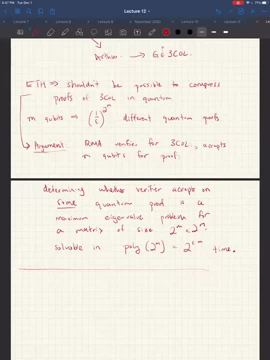 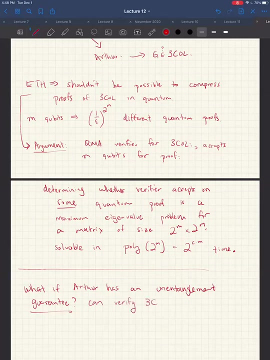 But if we now introduce an entanglement, an entanglement guarantee, then the story is going to be more information-consuming. But then the story changes dramatically. We actually get an exponential improvement in the proof sizes. So let's go back to the original example that we wrote. 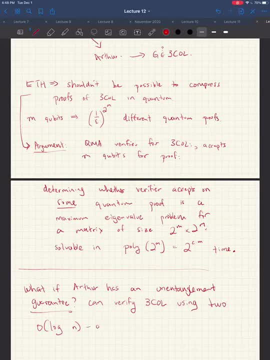 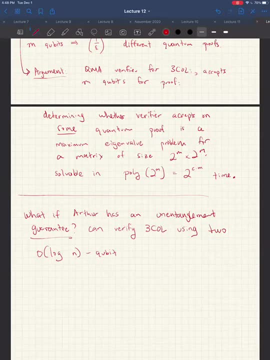 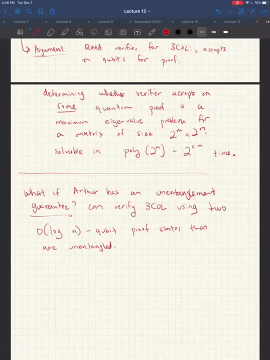 So, using two proof states of size order log n that are promised to be unentangled, he can verify three-coloring. Okay, so let's see how this works. This is a scheme that's due to Blea and Tapp. 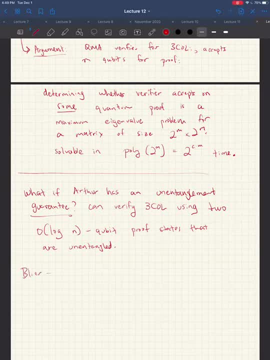 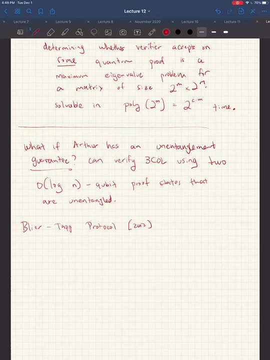 It's called the Blea and Tapp protocol. I think they came up with it in 2002.. It's a wonderfully simple idea, So let's fix an n-vertex, graph G, And then what Arthur is going to hope that Merlin will provide, as the proof is the following: 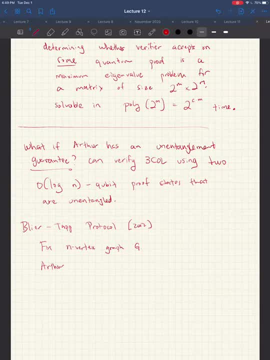 I mean, we don't know that Merlin will provide something like this, but let's just assume it for now. So Arthur hopes Merlin provides unentangled state of the form psi, tensor psi, where psi has the following format: So it's going to be a uniform superposition over all the vertices in the graph. 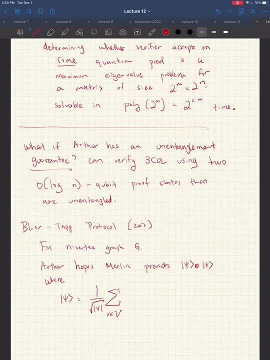 There's n of them And we sum over the vertices and we're going to have a register that corresponds of this proof. So this is going to be a V-register, So we're going to have one that corresponds to a vertex, vertex V- and we're also going 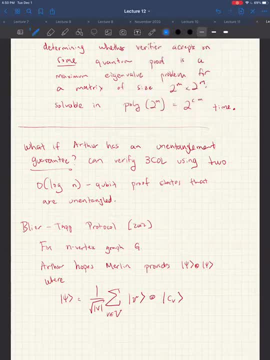 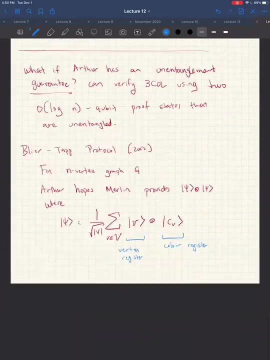 to have a register that corresponds to a supposed coloring of V. Okay, So this is going to be the call the vertex register And this is called the color register. And you know how big is this state? Well, it's about six centimeters in diameter. It's about four centimeters in diameter. So you have a three-shape or a six-shape distribution And then it's going to be a two-shape, And then it'll have a two-shape, And then it'll have a three-shape. 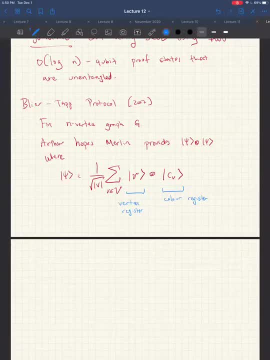 So the two-shape is going to be a half and half of two, which is kind of like an L-shape, And then it's going to have a two-shape. Well, it's log n qubits, right, Because to write down the name of any vertex, 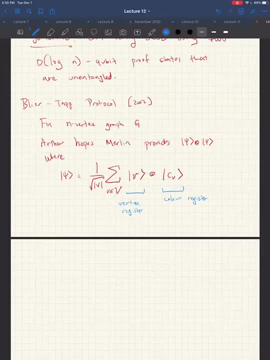 that's log n qubits. And the colors: well, there's only one of three colors, So there's a constant number of- you know, constant number of qubits to encode that. So in total it's log n- you know order log n qubits. 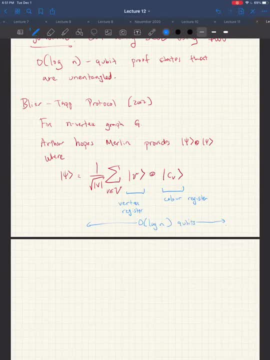 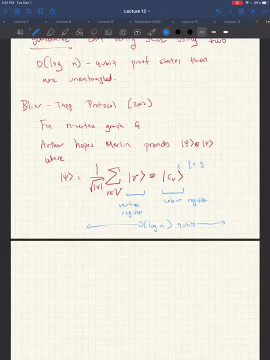 Okay, So Arthur is going to hope that Merlin provides state of this form And so this CV should be, say RGB, And Arthur wants to check that this coloring, the C, is a valid three coloring, Meaning that when you look across an edge, 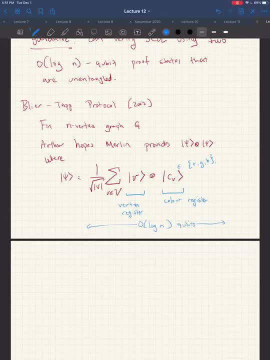 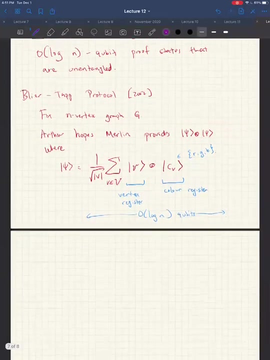 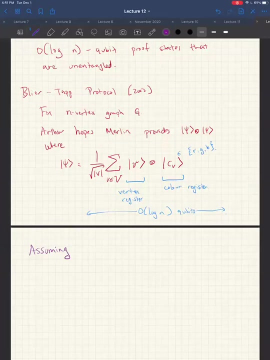 the two vertices at the end points don't share the same color. Okay, So how can Arthur check this? Let's see. let's use this color. So let's say that the proofs are really formatted in this way. So assuming proof is what I call well formatted. 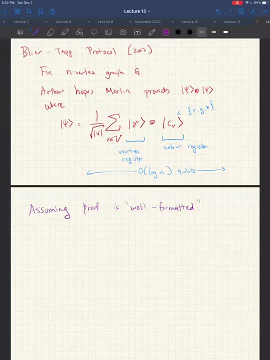 and we'll see how to verify this assumption. But what Arthur is going to do is Arthur is going to measure all. I mean there's two vertex registers and two color registers, right Cause there's there's side tensor side. Arthur is going to measure all of them in the standard basis. 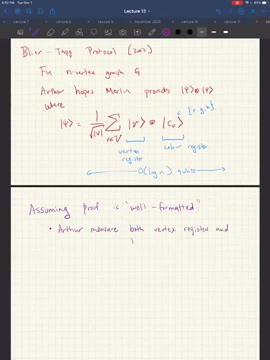 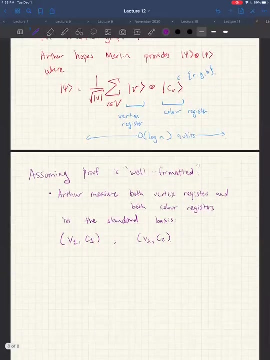 Both vertex registers and both color registers, All of the registers in the standard basis. And what does he get? Well, he gets two outcomes. So he's going to get vertex one- C one And vertex two- C two. And because these proofs are unentangled, 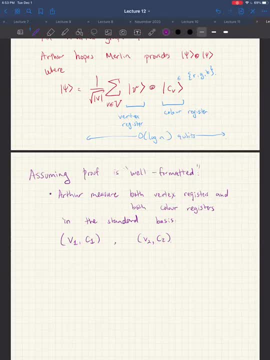 the distribution of V1, C1 and the distribution of V2, C2 are going to be independent and they're going to be uniform, right? So then Arthur's gonna look. Okay to look. suppose that v1 happens to be a neighbor of v2 in the graph, so if v1 and v2 is an edge, 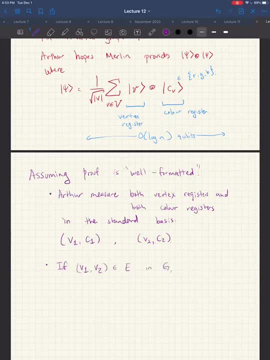 in g, then it's going to just look at the colors for these two vertices. if c1 is equal to c2, then that's really bad. so arthur is going to reject, but in all other cases arthur is just going to be happy with what's been given. 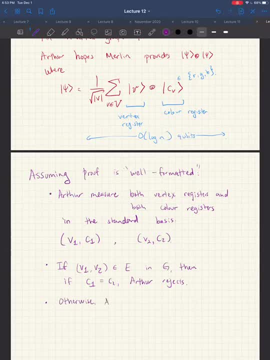 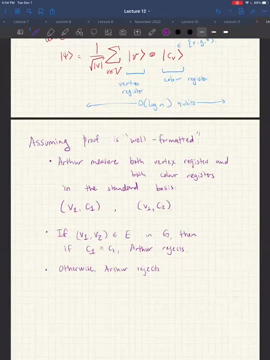 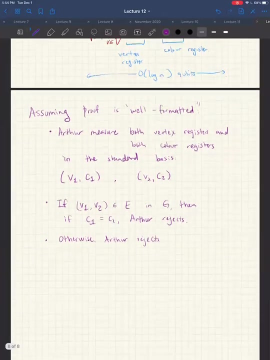 right. so basically in this, in this check, arthur is just going to sample two vertices and if they happen to be an edge, he's going to check whether the the coloring constraint is satisfied. if it's not satisfied, then he rejects, otherwise he's happy wait. so otherwise accept. oh, sorry, yeah. 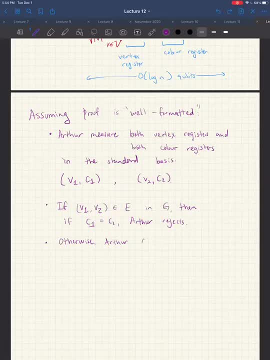 uh, no, he's, uh, yeah, otherwise arthur uh accepts, thanks, thanks, okay, um, so you know, uh again, just assuming that things are well formatted, we can think about the completeness and soundness of this proof system. so suppose g is three colorable, then What is the probability of acceptance? 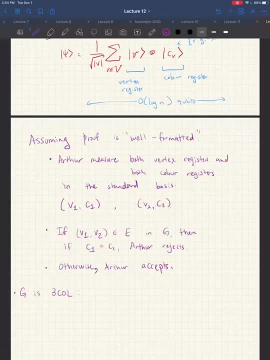 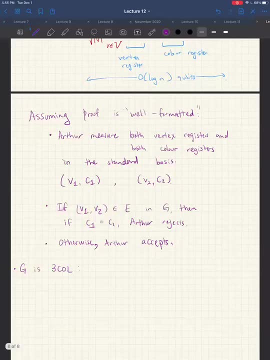 Well, Merlin will provide the proper coloring in these two proof states. They'll be well formatted And so whenever Arthur measures, he's never going to see inconsistent or he's never gonna see a violation of the coloring constraint. So he's always going to accept. 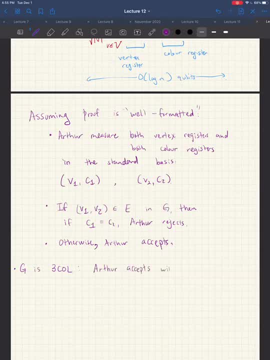 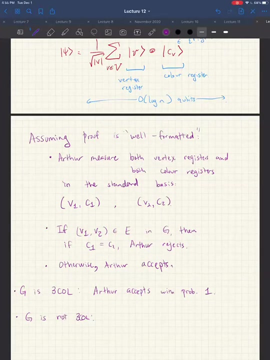 So Arthur accepts with probability one. Okay, so that's the easy case. What if G is not three-colorable? What happens So, since we're assuming that things are well formatted, we're assuming that Merlin has committed to some coloring of the vertices? 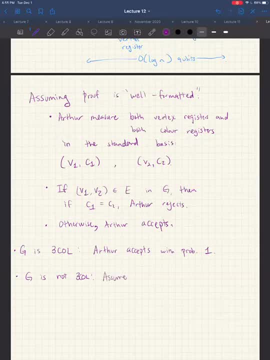 So- Well, there is going to be some edge which is mono, Monochromatic. He'll catch it with probability at least one over N squared. So any coloring violates the constraints in at least one edge. So, Arthur- you know, he's sampling two uniformly random vertices. 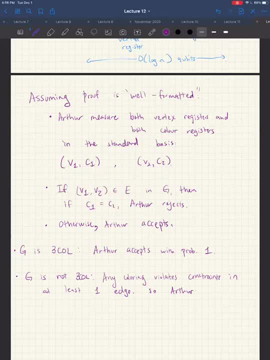 and with probability, you know, two over N squared or something like that is violated edge. it's probability, two over N squared and thus rejects, Thus reject, with probability at least: two over N squared, One over, sorry, two over N squared. 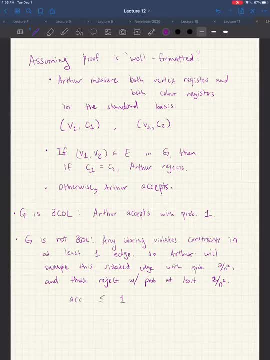 So, just putting it another way, the probability of acceptance is at most one minus one over two over N squared. So there's, you know, there's going to be a gap between the yes and no cases. It's between one and one minus two over N squared. 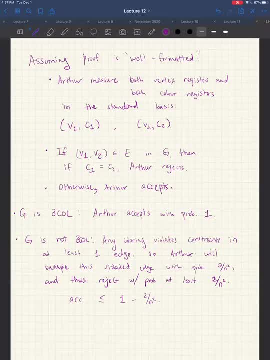 It's not a very large gap. it's an inverse polynomial gap And you know, we'll see how to boost this gap up to a constant later. I mean ideally you would like to say one versus one half or something like that. 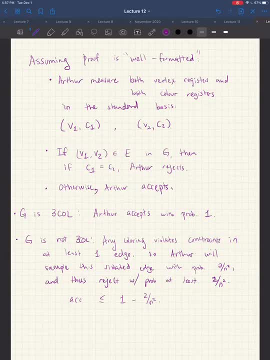 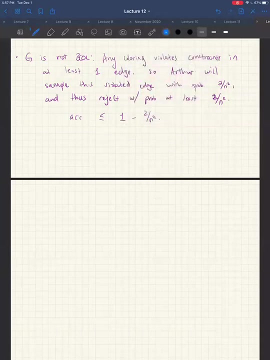 But before we get there, we still have this assumption that the proof was well formatted. okay, But we don't necessarily have that assumption. All that we're guaranteed is Merlin is providing a state of the form phi, tensor theta, So we're just guaranteed that. 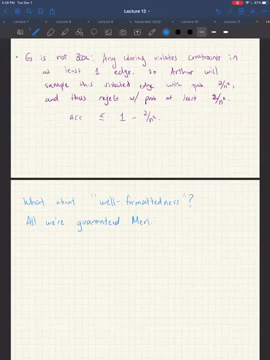 So we're just guaranteed that. Okay, so we just have these two unentangled states, both on order log N qubits. We don't even know that they're the same state, right? And so we have to do some checks, right. 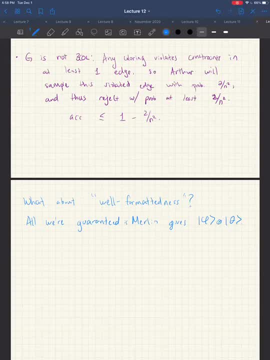 Okay, good, Let's see. So you know in particular this: you know for all, we know this state phi on the left, it could be some arbitrary superposition over vertices and colors. right, It can just look like you know for some. you know. 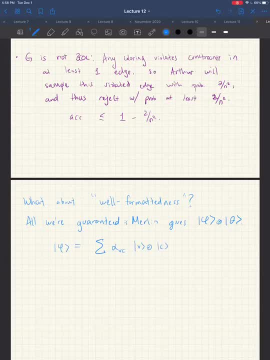 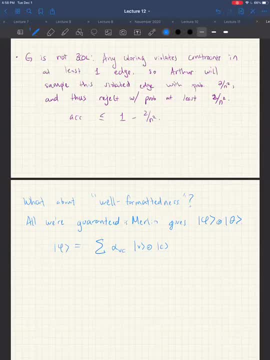 over the vertices right. Like a cheating, Merlin could try to say: I'm only going to put weight on the vertices that I know I can satisfy And furthermore, for each of the vertices it could put more than one color right. 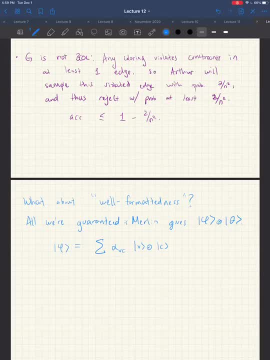 It could have a superposition of the colors right, And then it wouldn't be well formatted. So we're going to check that it's actually well formatted and we're going to have to introduce, to introduce, some additional tests. So really, the final protocol comes down to this. 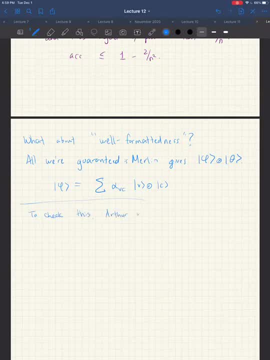 So, to check this, Arthur will perform one of the following tests uniformly, at random. So the first test? well, the first test is the coloring test, which we already saw. So this is from before. The other test is we're going to do. 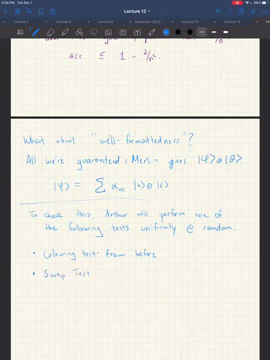 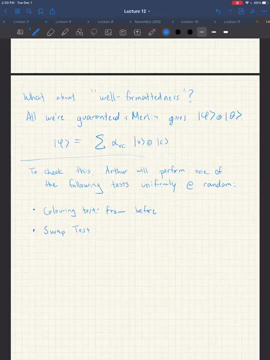 what's called a swap test. So this is where we're going to check that actually, these states are the same. So this is a test that you do on given two periods of time. So you do, let me make sure I get this right. 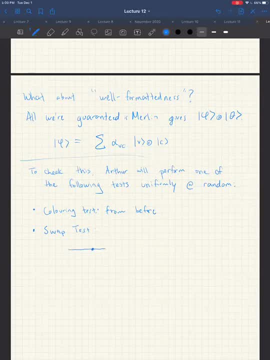 something like you have an ancilla qubit, I think. you start off in the plus state And you do a conditional swap on two pure states. So we have phi tensor theta And you do a conditional swap on two pure states. So we have phi tensor theta. 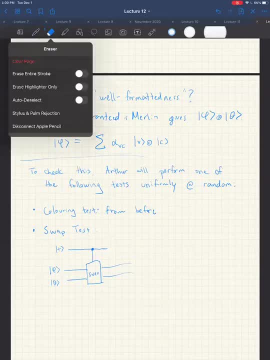 And you do a conditional swap on two pure states And you do a conditional swap on two pure states. Okay, Okay, And so so what this means is, if the top qubit is in the state zero, then you don't swap. 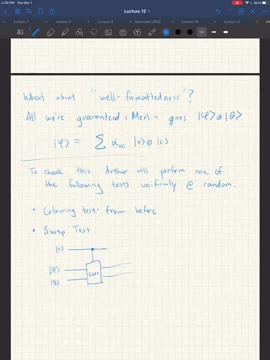 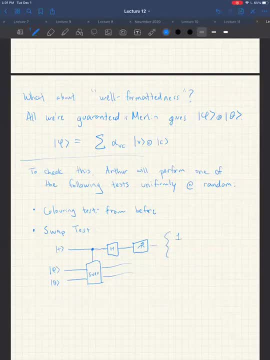 if it's one, then we declare: we think that phi is equal to theta. If it's zero, then we think that they're not the same. Actually, that's kind of confusing- Let me write it a different way- The probability that this circuit will output one. 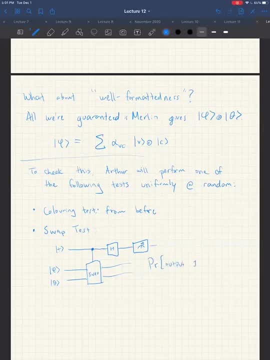 is equal to one half plus one half times the overlap between these two states. So case one: if these states are really the same, then this swap test will accept with probability one, And if they're orthogonal, if they're completely different, then accepts with probability a half, not zero, but a half. 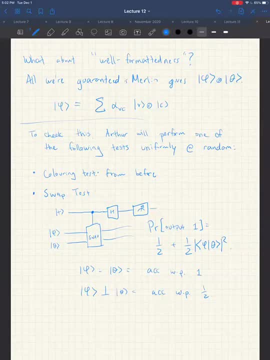 And then if it's somewhere in between, like it's in between orthogonal and being the same, then the acceptance probability will be somewhere between one half and one. The point is that it gives you some indication of how close these two states are. So by performing this test, the swap test, 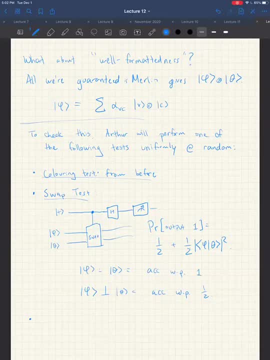 then basically we can guarantee to ourselves that phi is at least approximately close to theta, And that'll be good enough for us. Let's assume that they were the same. We want to now make sure that the state really looks like this uniform superposition over vertices. 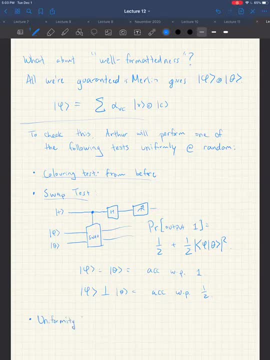 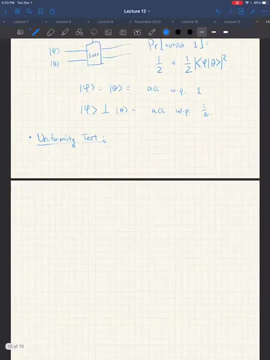 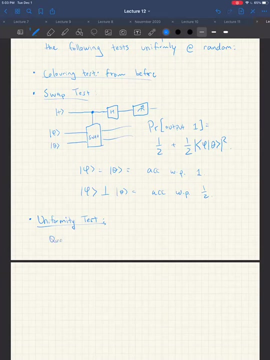 So we'll perform this uniformity test, And this is where you know the verifier is going to apply the quantum Fourier transform. So let's just quickly remind ourselves what the quantum Fourier transform is. So it's a transform. We specify what order transform we want. 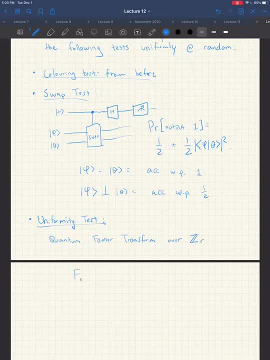 So let's say we want it over ZR. This is some unitary map, okay, And I call it FR. That maps an integer that's between zero and R. to this following superposition: Superposition over Y, which goes from zero to R minus one: 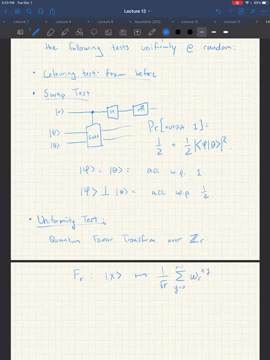 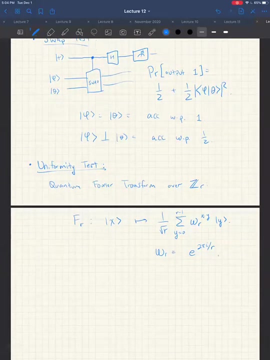 Then you have these Rth roots of unity. Okay, so hopefully this should ring a bell if you've taken a quantum computing class before. Anyway, it's it. It's some unitary map that looks like this. So what Arthur is going to do is: 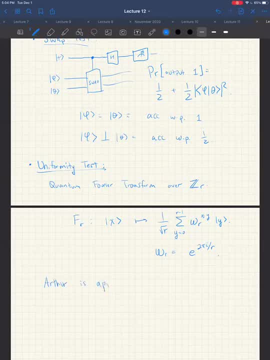 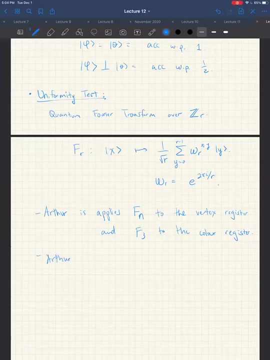 Arthur is going to apply F- what is it? Fn to the vertex register and F3, so it's gonna do two Fourier transforms to the color register And then it's going to measure both registers in the standard basis. So here it's just focusing on, say, P1,. 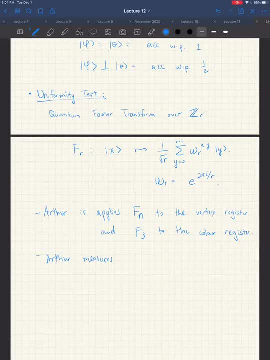 like the, we're already assuming that it's of the form Psi, tensor Psi. So because of the swap test, So we can just restrict ourselves to the first proof state, right? So we just have a vertex and a color register. So Arthur measures. 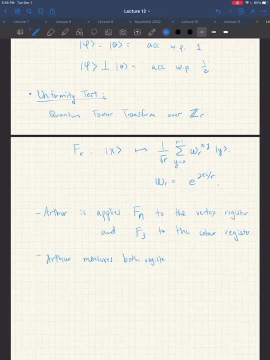 both registers in standard basis. If the color register happens to be zero but the vertex register is non-zero, then Arthur rejects. Otherwise, in any other case, we accept. Okay, so we won't go through the analysis here, but you can do the calculations. 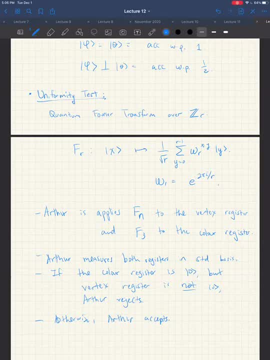 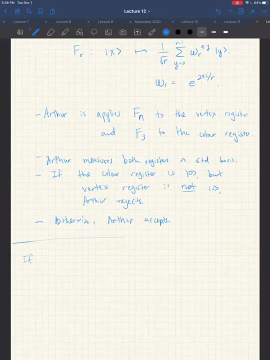 and you can see that if we pass all of these tests- the swap test, the uniformity test- then we've guaranteed ourselves that the proof state is well-formatted. So in the yes case, if the psi tensor psi is well-formatted, 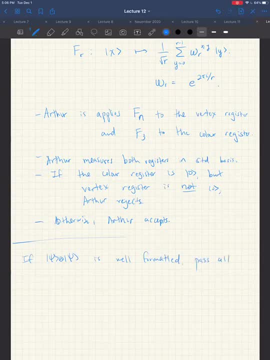 we pass all of these tests with probability one. And then, conversely, if we pass the test, if we pass the test with probability something pretty close to one, say one minus n, to the minus six apparently, then the state this: phi tensor theta. 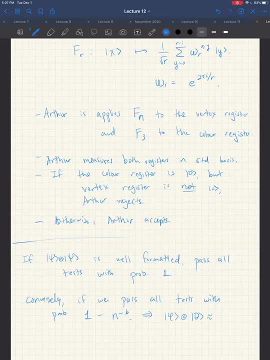 is going to be very close. You know how close It's going to be, like n to the, I'll just make up numbers here. but it's like n to the minus to. you know it's very close to being well-formatted. 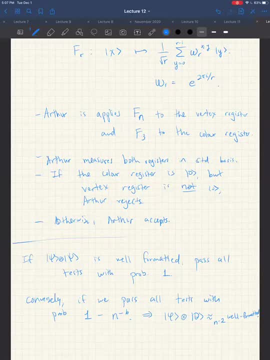 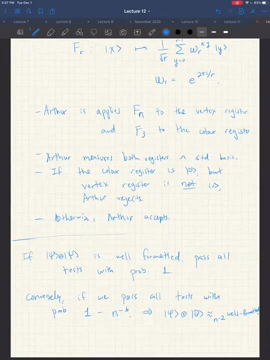 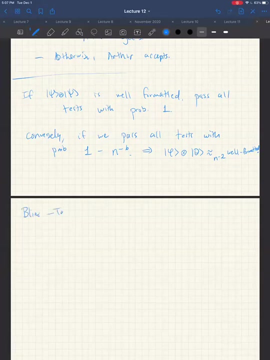 Okay, And then, once we know that it's close to being well-formatted, we can do the coloring test and everything will be fine. So this is like the conclusion of the Lie-Tap protocol. You know, in the yes case we have the probability one. 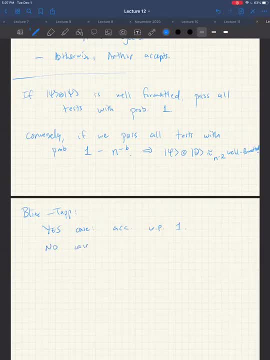 except with probability one In the no case you accept, with probability at most one minus n to the minus six. So so that's what the the difference between the soundness and completeness is. And there we have it. We have a protocol for. 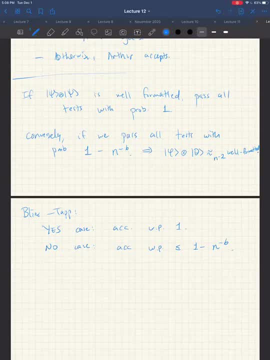 for very succinctly proving to someone using these log n qubit proofs that a graph is three-colonable, which is somewhat surprising. This proof is also like zero knowledge in some sense right, Like okay, if you assume that Merlin chooses some permutation beforehand of the coloring, which is cool. 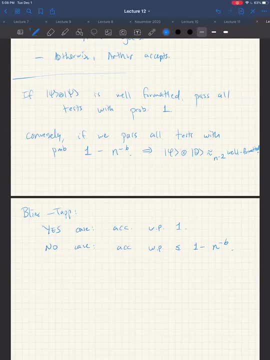 Yeah, that's a great. actually, that's something I've wondered about. I feel like there should be a way of I mean, yeah, inherently, it should be intuitively. it's like very, very, you know. 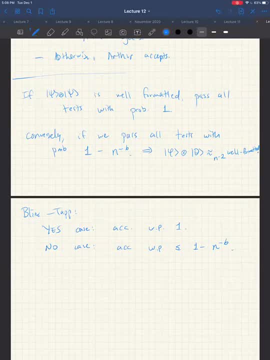 you have, at most, log n bits of knowledge, and then it should be easy to scramble anything inside of it. Actually, that's something that'd be great to work out. I think that'd be really cool. Nice, Yeah. so how about let's take a five-minute break? 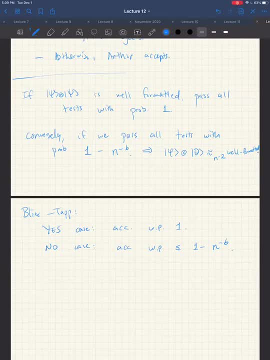 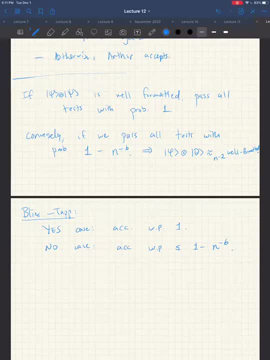 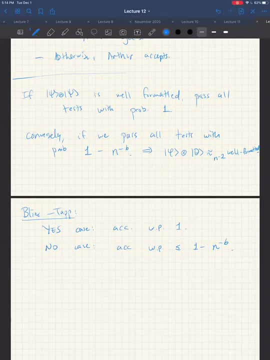 We'll be right back. We'll be right back, We'll be right back. I think one of the difficulty is that in zero knowledge, you have to handle any possible potential cheating verifier. So a verifier, even if he gets log n qubits, he could perform like an arbitrary measurement on it to extract some information. 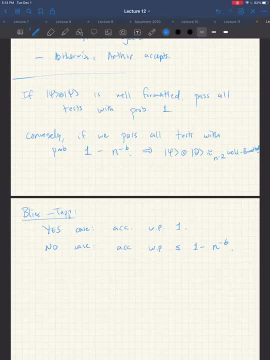 Yeah, And then you have to simulate it. It may not be clear, But maybe there's something there. I don't know, I'm just saying that it looks similar. yeah, no, no, I've had the same feeling. yeah, I think it's worth. I don't. I don't know if I don't think anyone's thought about it so. 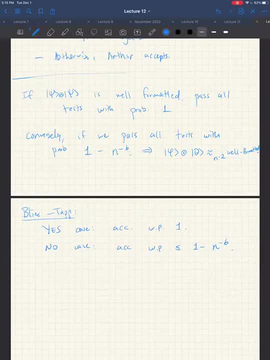 it might be worth thinking about. yeah, uh, okay, so, so let's, it's 5, 15, let's, uh, let's carry on, um, so, yeah, so we have this protocol, um, and it's, it's pretty cool, but, uh, you might be uh unhappy about this. this gap between the yes and no cases, it's very small. 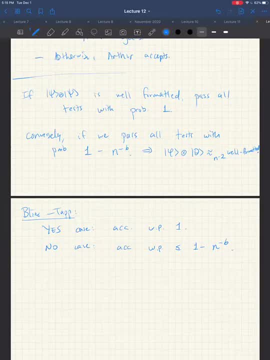 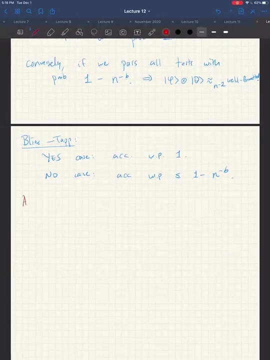 and you know, like if you see that in the protocol that Arthur has accepted, you don't have that much confidence about whether it's a yes or no instance. so ideally you'd like to amplify this gap. so, um, and you know, typically with a lot of these like models of randomized computation, like if 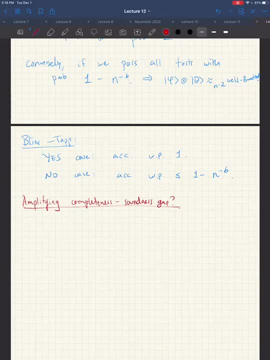 you have a randomized algorithm or like you know um, you know QMA or something. if the gap between the yes and no cases is too small, then you're going to have a lot of problems with the yes and no instances is inverse polynomial. you're not so worried because you say: well, I'll just repeat. 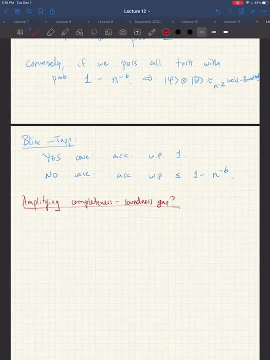 a polynomial number of times, uh, to boost my confidence up, and then you get a gap, that's say, a constant um. but uh, there's a couple issues, um, so you say you know why not? um, you know, repeat this BLEATAP, QMA2 protocol to boost the, the gap. 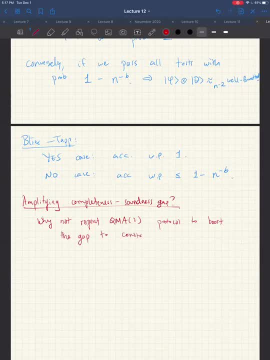 um, uh to constant. so, um, you know there's. there's two problems. one is that it's not known that by just repeating it in in you know the naive way, you just like run like a, a large number of instances in parallel. that'll actually improve the gap. this is, this is. 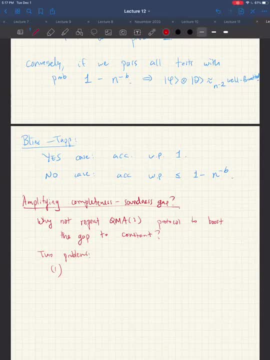 not unlike QMA. we know this is true. like, if you repeat the QMA verification process, um, you know a hundred times, you're going to have a lot of problems with the gap between the yes and no cases times. then the gap will, will you know, uh, increase by the the. you know the corresponding amount. 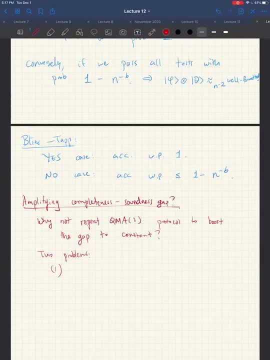 um, but, but we don't know this for QMA2. somehow this unentanglement guarantee sort of gets in the way. so it's unknown if parallel repetition will increase our confidence in the usual way. but even if it did, we're still. we still have another problem. 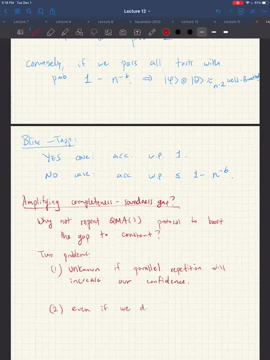 um, like, may i ask, like, what is the what, what is the bot of the bottleneck? because, like you, just sample more and more edges, so probably probability to fall on that edge, which is monochromatic, is small. smaller unless somehow the- uh, the malicious prover can somehow choose different. 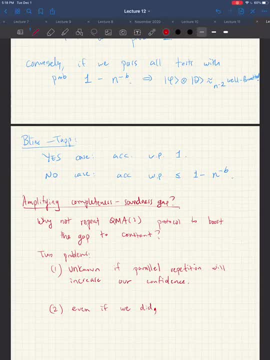 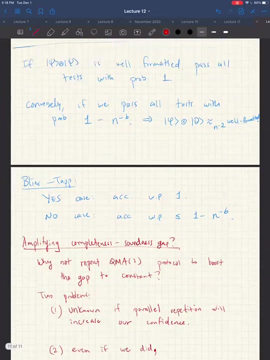 colorings each time, or some some something. yeah so, um, you know, the the verifier is not just doing this checking the coloring, it's also doing this uniformity test. yes, so these tests, uh, oh, the thing to know, that's a good question. the thing to notice is that they're they take these two. 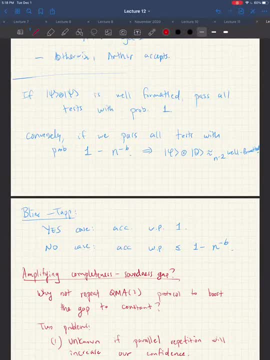 unentangled proofs and they'll do something to get them jointly and they'll actually entangle the proofs together in some weird way. so so now you imagine if um Merlin now provides you with, supposedly, a bunch of copies of these uh states when you do these um 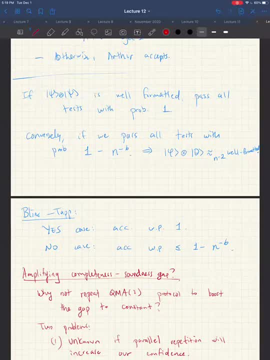 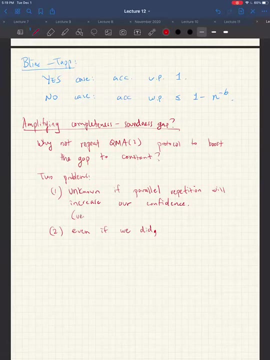 these, uh, these like uniformity and swap tests and things. you actually introduce entanglement between the two copies and then you're no longer guaranteed to have this unentanglement guarantee. so yeah, let's write a note there. verifier, could you know, inadvertently break the unentanglement guarantee. 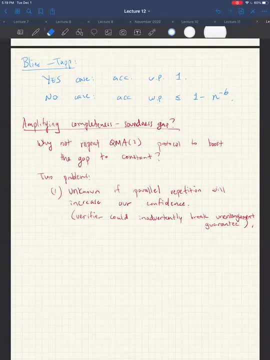 right, which is a very precious thing for us- that we would like to maintain that. um. but number two, like even if parallel repetition did work, uh, we still have this issue, at least with this Blea-Tap protocol, which is that the gap between the yes and no instances is n to the minus six. so how many? 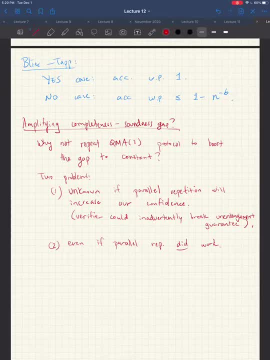 times would you have to repeat the protocol in order to um, in order to, you know, boost your confidence up to a constant? you would think n to the six times, but you know it's not always the case, um. but but then that would sort of be pointless, because then your proof sizes are. 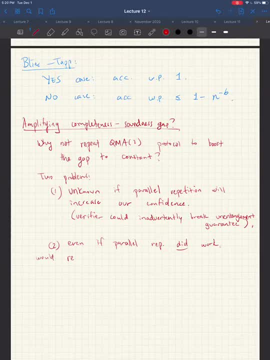 you know, uh n to the six times larger. so you've wiped out any of these savings from having a compressed proof, right? so I think we just need to make sure that that's the case. um, so you know, for each one we have to do something a little bit harder. 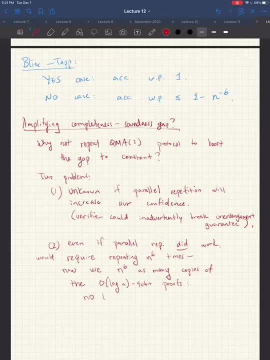 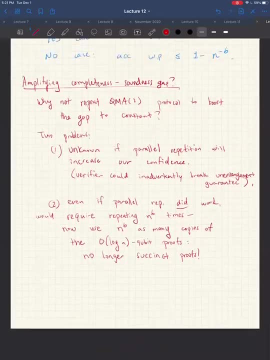 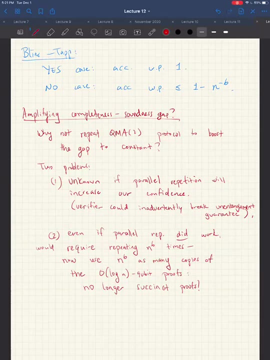 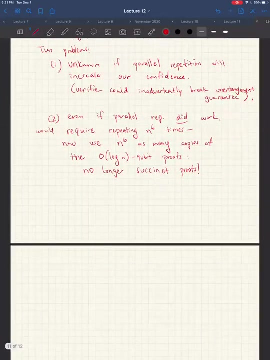 than what we do exactly. do something just flatter than, or just D. so you know, it seems like we're we're kind of stuck, um, or at least you know we have to do something a little more clever. um, It turns out that you can boost the soundness in this gap. 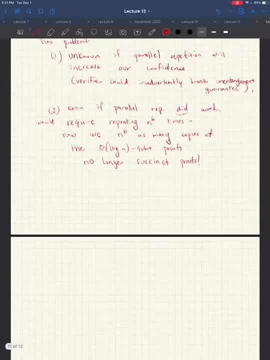 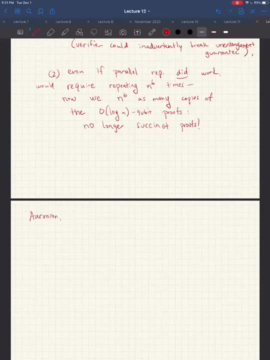 And this was done in a couple of follow-up papers. So there's a paper by Aronson Begge, Drucker, Pfefferman and Peter Schor. And what do they show? They showed that you can create a. 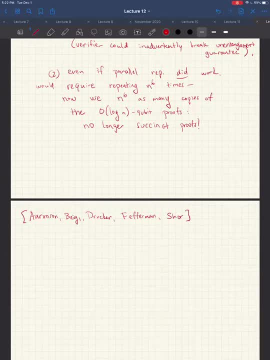 not a QMA2 protocol but QMA-M protocol with basically have many more unentangled proofs. So they created a protocol for 3SAT, not 3-coloring, for 3SAT instances of size M, right, So I guess the size of a 3SAT instance. 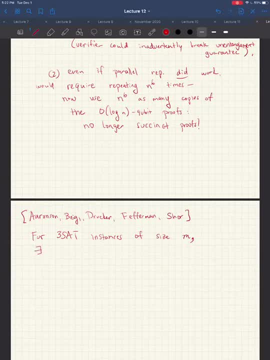 is like the number of variables plus the number of clauses. There exists a QMA-M protocol, So this is where you have a stronger unentanglement guarantee. So this is where you know Merlin is going to give you M different registers, so P1, P2, up to PM. 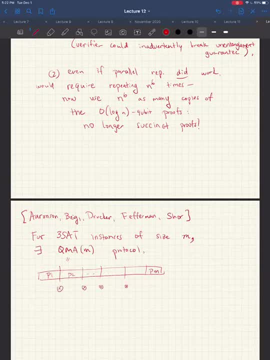 and they're all going to be unentangled with each other. And then they start to show up in your protocol, and then you have to provide them with a 3SAT extension, And then you have to provide data to the first instance of the extension to show that you have a stronger 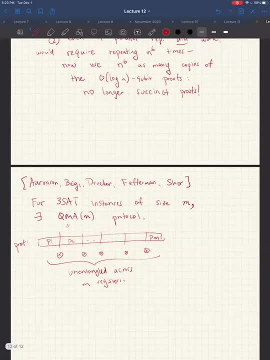 unentanglement guarantee. So okay, so you know, there's this extension where you have a stronger unentanglement guarantee, There's a QMA protocol where, oh, oh so Sorry, I think I kind of messed up. 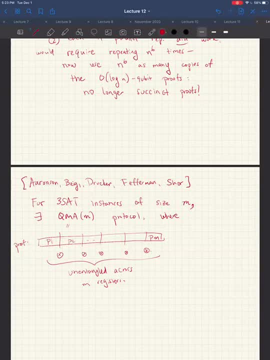 It's not the number of registers here is not M, because M is the size of. let me call it K QMAK protocol. So there's K parts to the proof, And how big is K? K is going to be equal to square root M. 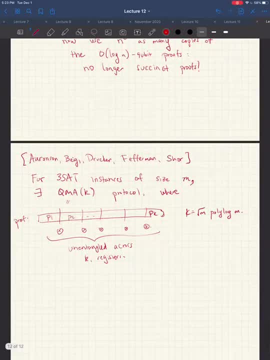 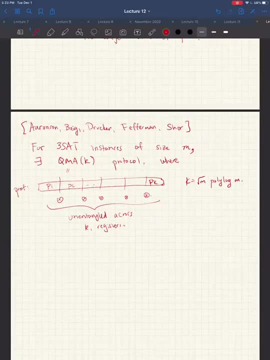 poly log M. okay, So there's going to be square root M, roughly square root M, unentangled proofs. How big is each register? Each register is still log M qubits And using so in you know how many qubits is this total? 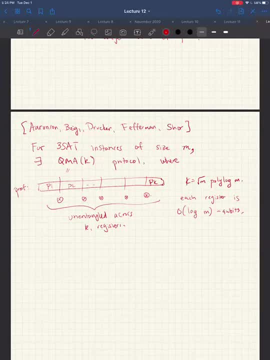 It's going to be square root M times poly log M. Very visit, very good. I'm going to call this the 50th instance And this is going to be the last one, because I don't want to go back and look at it again. 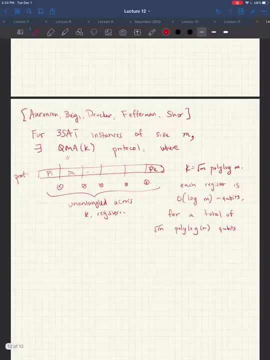 So I'm going to call this the 50th instance and I'm going to create an element here to say that I assume that this is the final result. So this is the final result of the liverization, And I'm going to say: 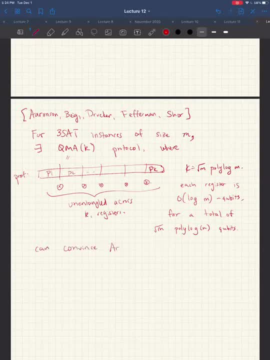 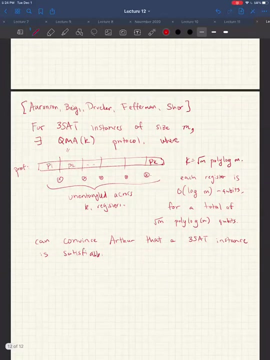 I assume, get- and I'm going to call this the 50th instance. There are a few more exist in terms of this, but that's a good thing. okay, We'll see. So again, we're getting some compression in the size of the proofs. 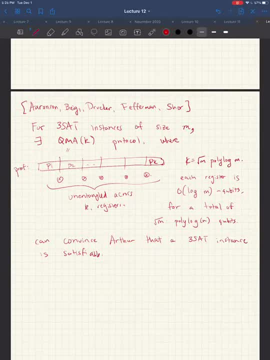 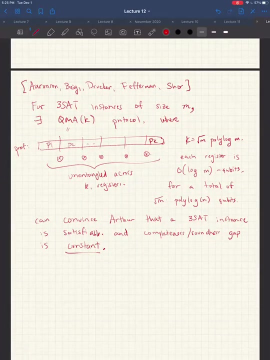 And furthermore, the completeness soundness gap is a constant, So it's no longer such a drastic savings. it's not going from n to log n, it's from n to square root n, but there's still some compression and we have this good confidence. 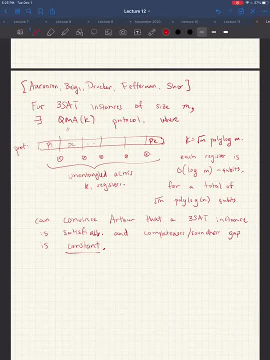 when we're doing this verification. There's this catch that I guess. now it looks like we need to assume that Merlin is giving us many unentangled chunks, not just two states. So the protocol is a lot more sophisticated than this Blier-Tap one, and I'll just say 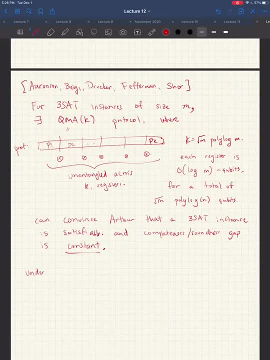 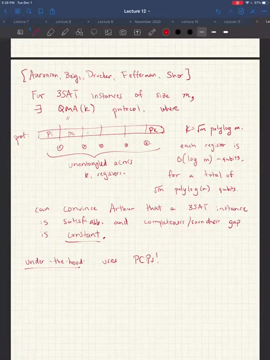 a few words about it. So what goes on under the hood? And it uses something we've heard before, which is PCPs. So this PCP keeps on making an appearance throughout this course, and this is no exception. The idea to use PCPs in this setting is quite natural, though. 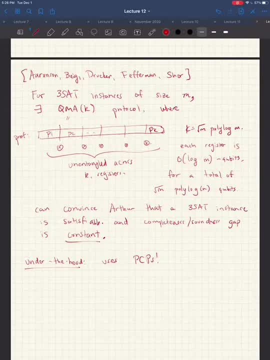 So one of the reasons why this Blier-Tap protocol has such a bad gap is because, in the no case, this graph is not three-colorable. We're only guaranteeing one. We're only guaranteeing that there's one violation lying somewhere in this graph, right? 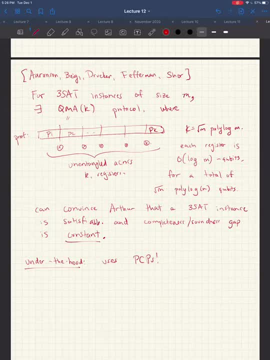 It could be that almost all of the edges are satisfied except for just one. So in order for Arthur to detect something wrong about this graph, it has to get lucky and locate exactly this one bad edge right. But what would be much nicer is if we somehow knew that this graph, if it was satisfiable. 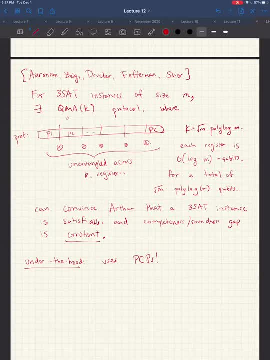 then of course all the edges would be satisfied. Right, Right, Right Right, All the edges are satisfied. But in the no case, if it's not satisfiable, we would hope that many, many edges are violating the coloring constraint. 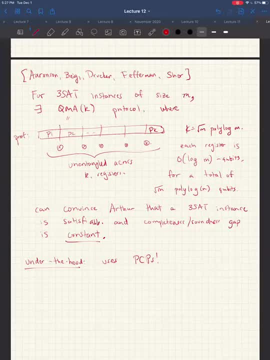 And PCPs are exactly this tool that allows you to get this. So PCPs allow you to take an instance. You can take an instance of your favorite NP-complete problem, let's say three-coloring. So it turns out that you do this transformation. so this PCP says: I'm going to get a new graph. 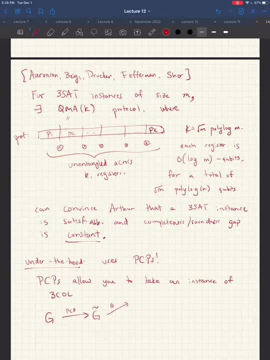 g prime, where if g is three-colorable, then so is g tilde. g tilde is also three-colorable. So if g is three-colorable, then so is g tilde. g tilde is also three-colorable. So if g is three-colorable, then so is g tilde. 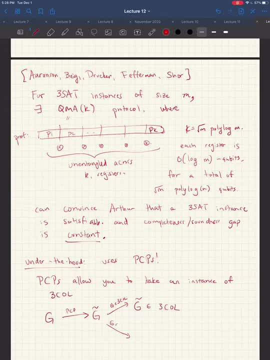 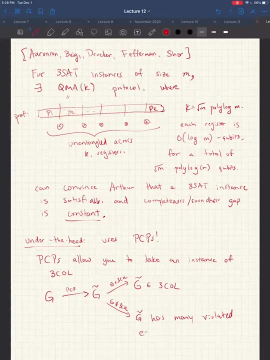 g tilde is also three-colorable. So if g is three-colorable, But if g is not three-colorable, then g tilde has many, many violating edges, In fact, a constant fraction. So this is what PCPs allow you to do. 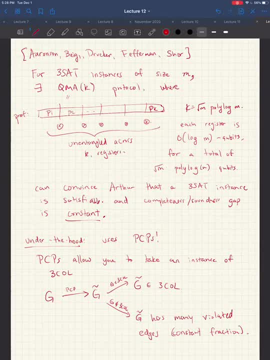 And if you have this guarantee, But if you have a seguirн or tar doesn't have any violating edges, then by just sampling it at random, will have a very good chance of finding the 2014 Ihab Foight Rodent violation. 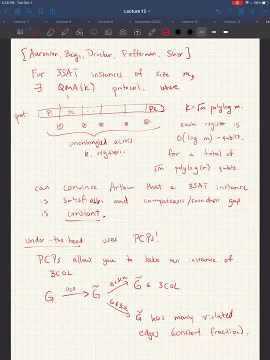 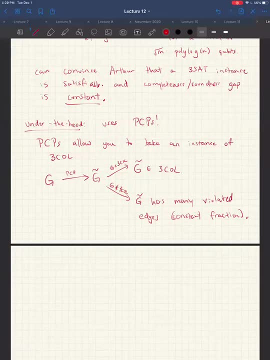 So that's kind of the starting point. Arthur, just by sampling it as uniformly at random, will have a very good chance of finding a relation. I mean, there's a lot of technical things you need to do to to get this ID to work. 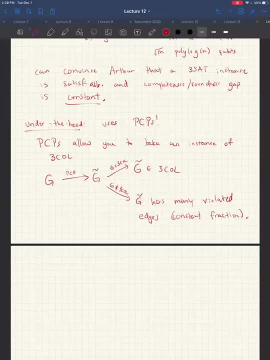 but really, at the heart of this is: you're really using this PCP. OK, so that's really cool, And you know. the final thing that you might be wondering about is what's the best way to use a PCP? Is it likely to find the 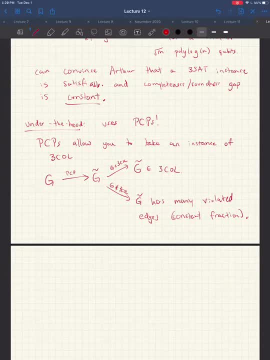 Okay, so that's really cool. The final thing that you might be wondering about is is: how essential is this stronger unentanglement guarantee? Now, is it essential that Merlin sends square root M unentangled proofs? And the answer is: it's not essential at all. 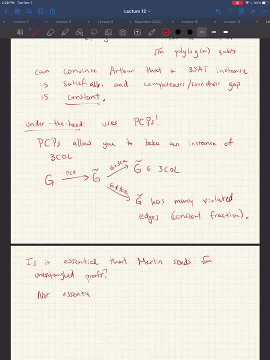 You can actually convert this protocol of Aronson et al into a QMA2 protocol. So you can. you only need to assume unentanglement between two registers, And this is captured by the fact that QMA k is equal to QMA2 for all. 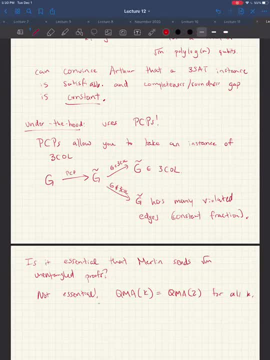 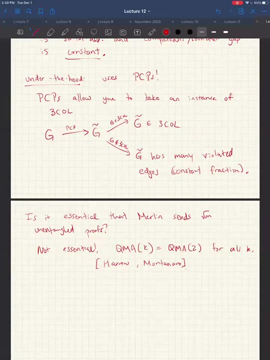 k And this was a. it's a result that's due to Harrow and Montanaro. So basically, as you know, from a proof verification point of view, there's no difference between having an unentanglement guarantee between many registers. 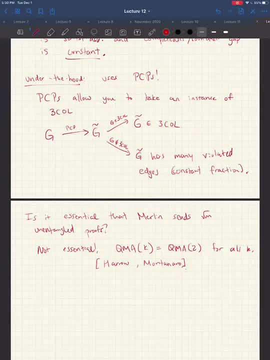 and a guarantee between two registers. Wait, you mean k larger than two, right? Oh, Oh, yes, yes, yes, yes, yes. K larger than two? yeah, Yeah, it's not known to hold for one. That's the big open question. 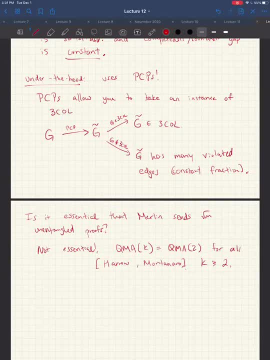 And even for like unconsonant K, Yeah, Poly, you know yeah. So, in particular, we don't know the relation between like QMA2 and IP2.. QMA2 and IP2? Like AM, to be precise. 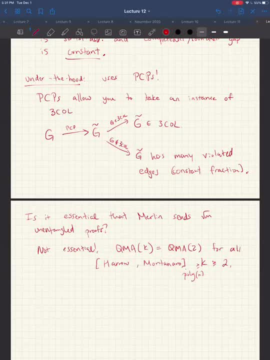 Oh Well, not necessarily AM, because I'm not saying that you need the randomness to be public. so IP2, yes, Yeah, I don't think we know what the randomness is. Yeah, I think that's an open question. 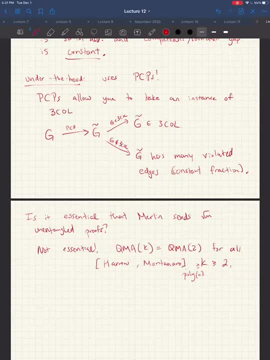 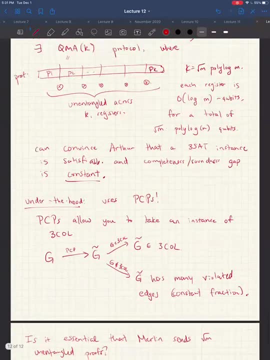 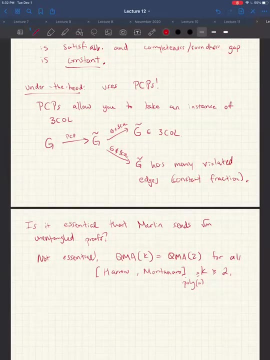 Yeah, Okay, Yeah, any other questions about these protocols? Yeah, could you elaborate a bit on how you go from G to G, tilde? I mean using the PCP. Oh, Oh, I mean that's. I guess there's a couple ways of answering that question. 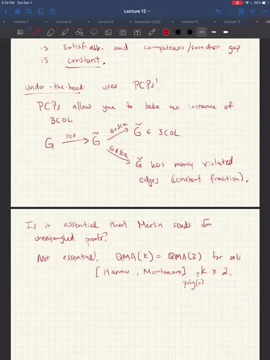 One is- you know before I've talked about PCPs, as, oh, you can check the validity of a proof by sampling three random locations. What does this have to do with this? converting a graph to another graph? That has to do with this. 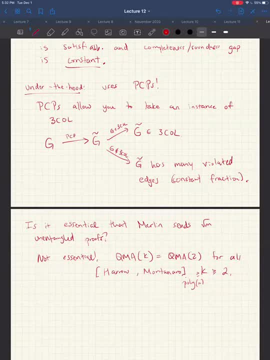 this equivalence between the hardness of approximation, of MP-complete problems, Oh sorry, of constraint satisfaction problems, and this proof verification which we kind of talked about before, And so that follows in a. well, let's see, I mean, I'm familiar with the hardness. 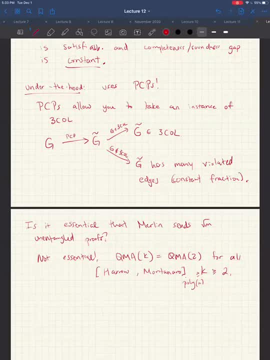 of approximation stuff. but still, even if I grant that, how do you construct this here to there? I see, yeah, That I don't know, off the top of my head I think maybe it's not black box. I think it's true, but yeah. 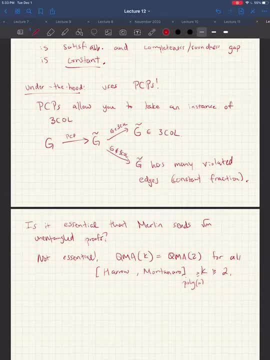 maybe I have to look up the reference, Right, yeah, Maybe, okay. so what I know for sure is that if you replace three coloring with three set, what I've written is certainly true, but I guess three coloring- it's maybe not immediately obvious. 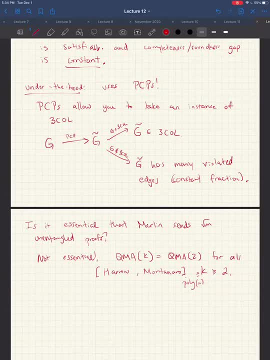 Yeah. So I have a question just about this last point here, about the essentialness of these unentangled proofs, the root M there. So, okay, it's not essential, but what is the motivation for root M Like? what's the intuition that they have? 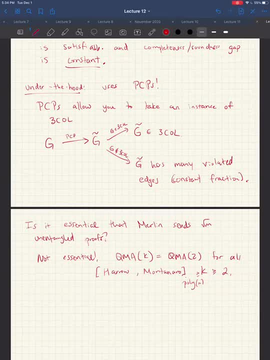 when it shows up that specific value. I was trying to understand the-. Yeah, why does root M pop up? That's a good question. Actually, it comes from using the. I think it comes from the birthday paradox. You know what's the birthday paradox? 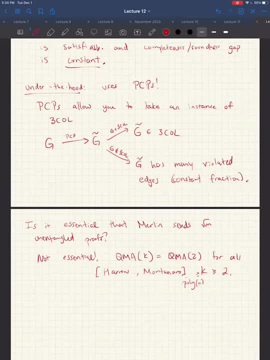 It says that if you're in a room with M people, you know what's the probability that you know two people in that room will share the same birthday. You know it's gonna be, you know square, you don't actually need that many people. 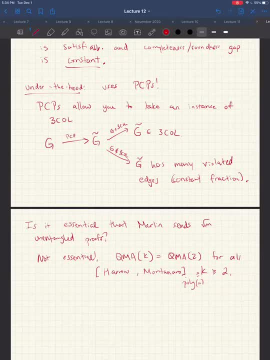 It just needs to be square root of 365 days before that happens. So that's kind of the same phenomenon that happens here. Basically, you can think of your sampling, you know. let's say you have M edges in a graph, right? 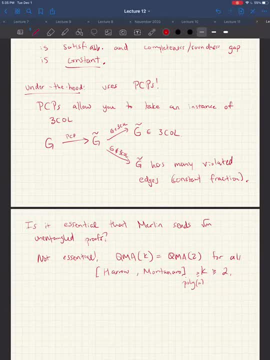 And you want to sample, you know. so you sample these edges uniformly at random. How many times do you need to sample them before you get a collision? You only with high probability. you only need to sample like square root M times. 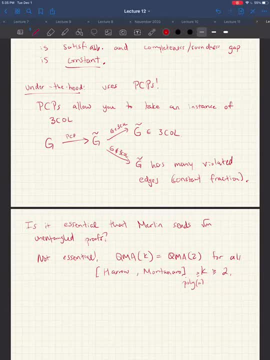 So that's one of the things that goes into why square root M is the right answer here. So it's like if you consider the graph to be co-expanded by some sort of square, it's like going the length or going the breadth of that square. 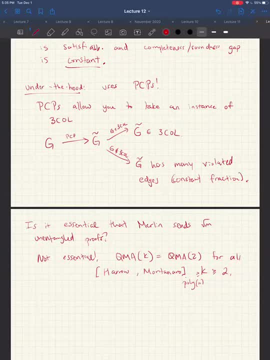 is a rough look down for how much you would need to traverse a graph in order to hit a collision. I guess right. So this has? yeah. well, this doesn't rely on the graphing of any particular shape, It's really just like yeah. 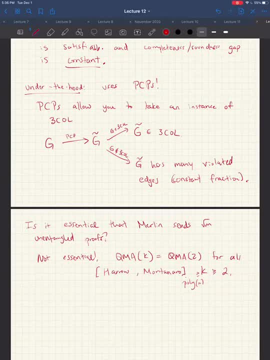 Okay, it's my own sort of mnemonic, Okay. so let's go to. so, you know. so this proof compression of, you know, having shorter proofs for 3SAT and 3-coloring, you know it's pretty fun. 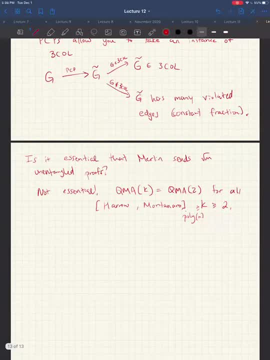 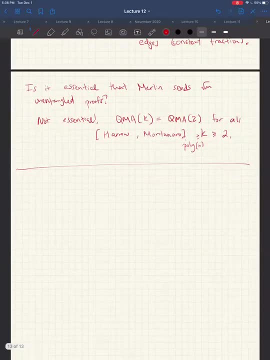 But you know there's more that we can. you know there's more reasons why this QMA2 complexity class is interesting And it has to do with connections with this complexity of detecting entanglement, In particular mixed detecting, mixed state entanglement. 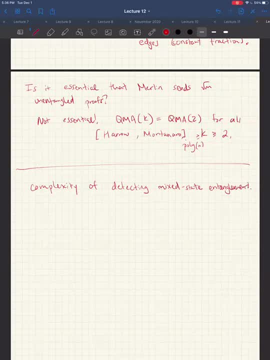 All right, so you know the motivation here is. you know, suppose I give you a classical description of a quantum state, right? So I just write down, like the vector or its density matrix. You tell me if it's entangled or not. 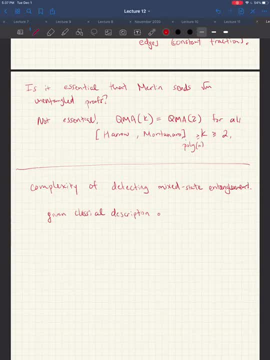 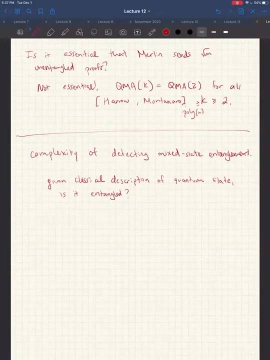 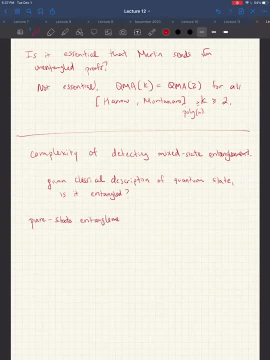 it's pure state entanglement, Right? so let's say that someone walks up to you with a vector you know in in CD tensor, CD, right, And it's not given to you in quantum form, but they like just write out this. 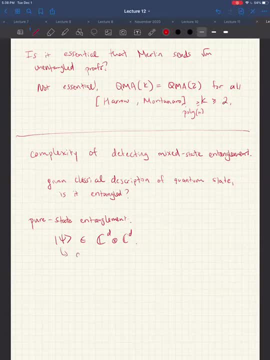 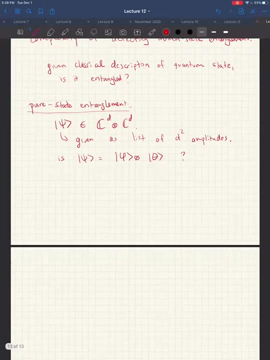 this list of amplitudes of size D squared. All right, you know how hard is it to you know determine whether psi is equal to phi tensor theta. How long would this take? Any, any, any ideas? Worst case, you'll have to go over. 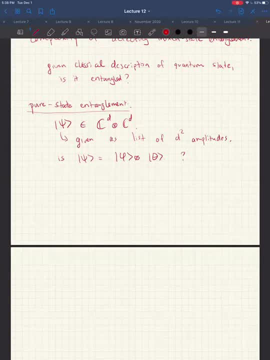 all the bipartitions in gold. Oh, oh, let's say sorry, I should have said I specify a bipartition. So yeah, with specify, specify by partition, right? So I tell you, here's registers P1 and P2.. 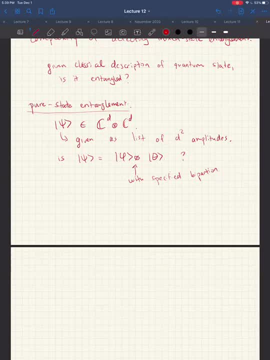 Is psi entangled across this partition. So how hard or easy is it then? I just have to calculate the trace, So like partial traces, right? Yeah, that should give you this information. Yeah, that'd be one way of doing it. 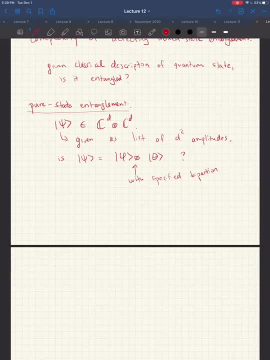 So in some sense, in some sense we consider this to be an easy problem. It only takes polynomial time in D, Only takes probably D time, right And and you know. so one way is you can take the partial trace. 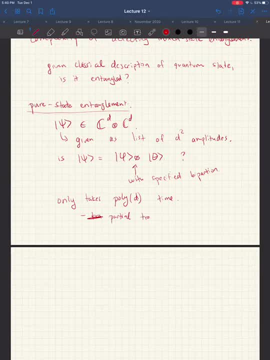 or you can compute it numerically, right, Or you know another way to do. it is: you can solve a linear system of equations, right? Your unknowns will be these two states Solve well, I guess it wouldn't be linear, but 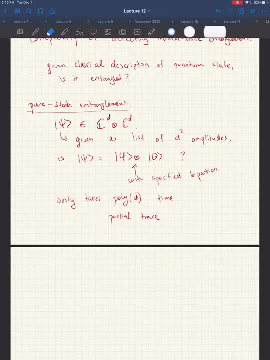 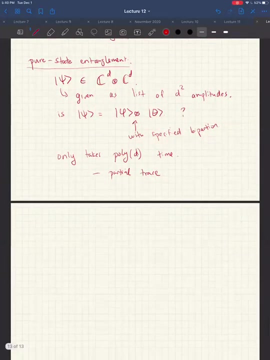 Actually, yeah, you should just do the partial trace. Yeah, so you can take the partial trace and just check that the, you know, the reduced state on one side is a rank one density matrix. So you know. so this is considered easy, right? 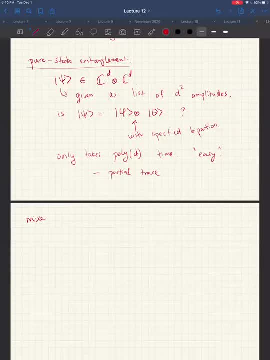 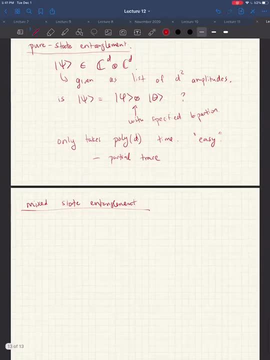 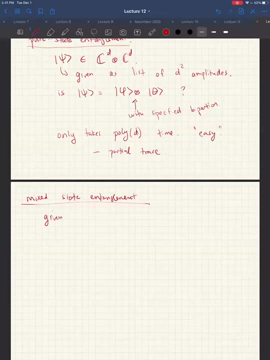 Polynomial time. But what about mixed state entanglement? So there the story is a little different. So let's say we're given a classical description of a density matrix on two registers. So given density matrix row on two registers, let's call them A and B. 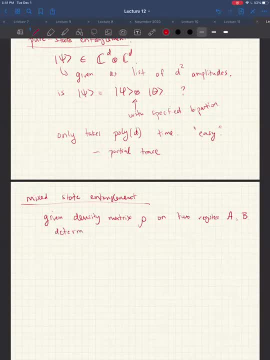 determine whether the state is what's called separable, What is separable? It's a state that's called separable because it's a state that's called separable. because it's a state that's called separable, So it's a state that's called separable. 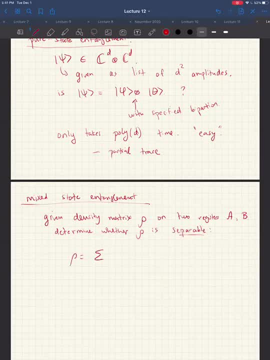 What's separable mean? It means that it's equal to a convex combination. Okay, so this is PI. This is a probability of a tensor product of two density matrices on registers A and B. So these are density matrices on A and B. 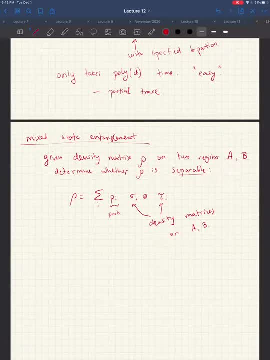 Okay so, and let's say that the dimensions of the registers A and B are also D, So this is dimension D, right? If a state is separable, it's not considered to have any quantum entanglement, So so this state is unentangled. 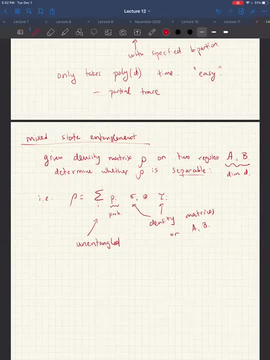 even though it might have correlations, classical correlations between the two registers, A and B, right, and the classical correlations only come in through this, this probability here. So, in particular, if you have a separable state, you cannot use it to win a non-local game. 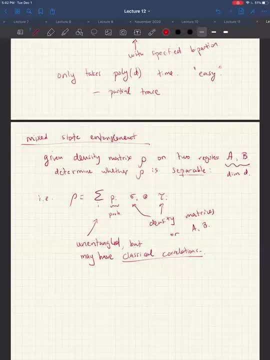 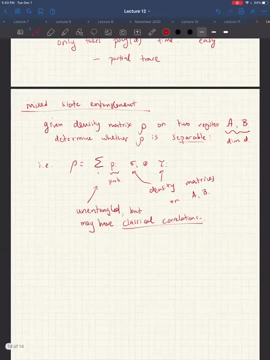 with higher than classical probability, for example. right, You cannot do anything essentially non-classical, roughly speaking. So okay, But someone hands you this testing matrix row. I mean it's specified as a. you know it's a D to the fourth by D to the fourth matrix. 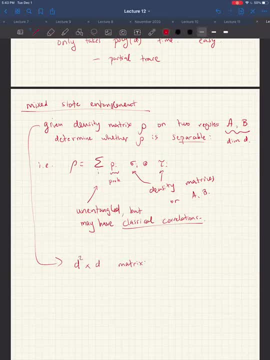 Sorry, D squared by D, squared right, Because that's its dimension. Can you tell whether it has this? it could be written in this mixture, right, And this looks to be like a much harder problem. So this is called the separable states problem. 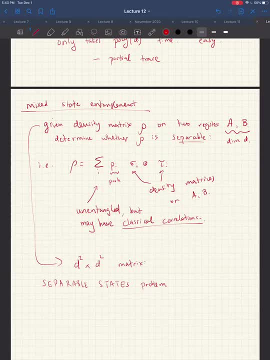 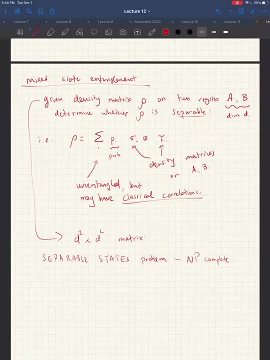 And- and this actually turns out to be an NP complete problem in the worst case. Okay, this was shocked. How do I solve this correct? So, when we got inside of the shell, athletics came in as the key ingredient To solve them all. 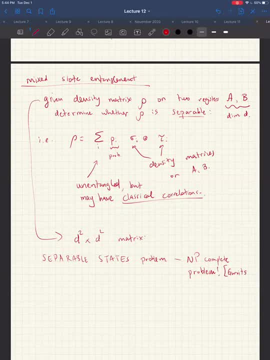 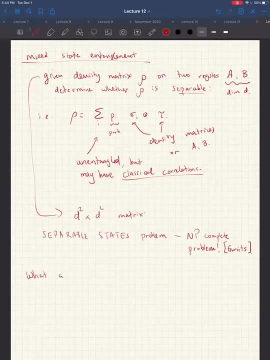 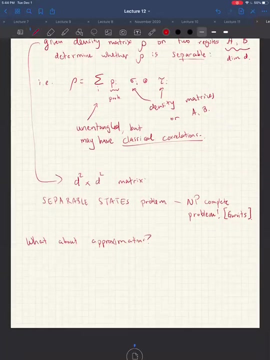 as shown by Gervitz. Okay, so in the worst case, to tell whether a density matrix row is separable, exactly this is NP-complete. But what about approximations? So we can think of the you know in density matrix space. 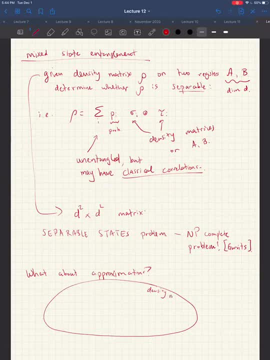 So you know, let's say that this is a set of all density matrices. There's a subset of them that's the separable state. So let's call this state SEP, And it turns out that the SEP is nice in some sense. 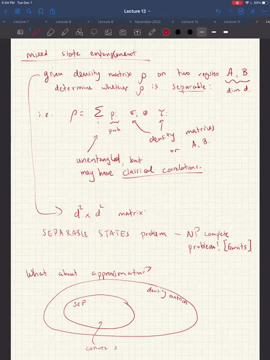 because it's a convex set, right, And you can see this because, by definition, separable states are convex mixtures of, you know, these tensor product states. And we're given some point row And we wanna know: is it either in the set? 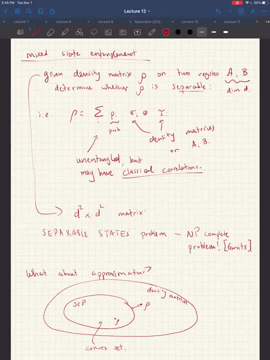 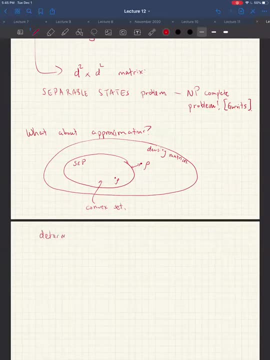 or is it far from the separable states? right Promise that one is the case. So we wanna determine if row is in the set of separable states or row is epsilon far from SEP, And this is one of the biggest open problems in quantum information theory. 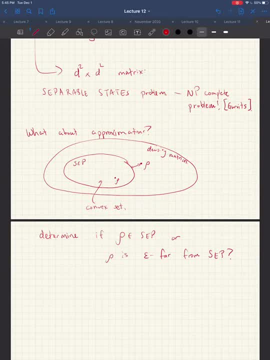 for whether there's an efficient algorithm for this approximation problem. So some people speculate that there's what's called the quasi polynomial time algorithm for this. So here's a speculation, and this is only some folks. people are divided on this. Maybe there's a quasi polynomial time algorithm. 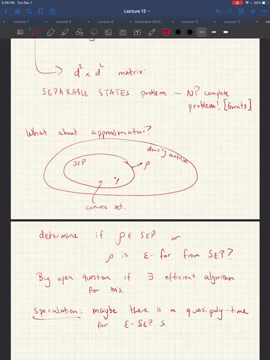 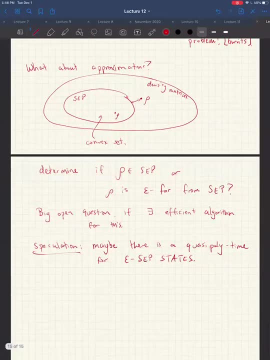 for what's called epsilon separable state. So epsilon is just some fixed constant like one 10th or 100 or something like one over 100.. By quasi polynomial I mean that it runs in time D to the poly log D time. 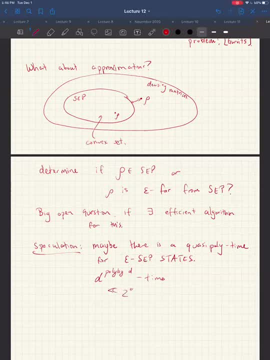 Okay, so it's not quite exponential. This is much, much less than two to the D, but it's also bigger than any polynomial. So that's why they call it quasi polynomial time, And then others conjecture that actually you need something closer to exponential time. 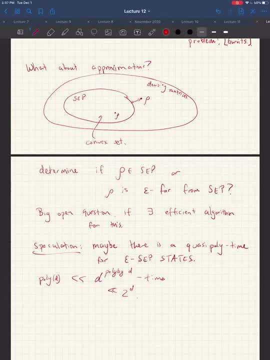 in order to determine whether a state is separable or not. But nobody really knows. But whether it's quasi polynomial or exponential time, I think most people believe that really detecting mixed state entanglement is a much, much harder problem than pure state entanglement, which is rather curious. 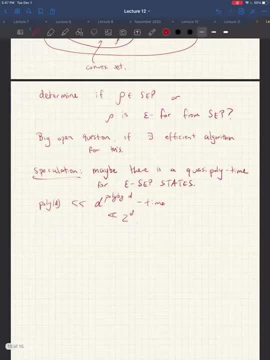 Now here's where the connection between this separable states and QMA2 comes in, which is that right now, we have very little idea about what the complexity of QMA2 is. So if we were to draw the complexity landscape, we have our class QMA right. 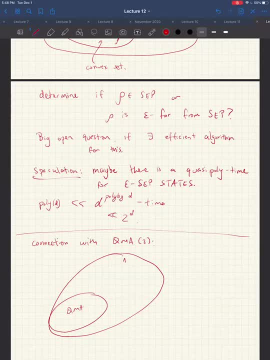 And then the best complexity upper bound we have for QMA2 is non-deterministic exponential time, right? Which is this? remember, it's like the complexity of solving exponentially large NP complete problems, Right? so we heard about that before. 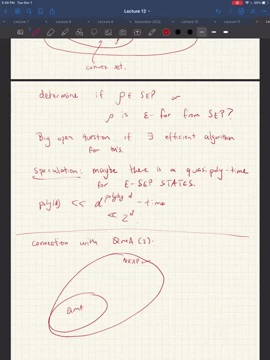 You know it's harder than exponential time and harder than polynomial space and so on, And QMA2 is anywhere in between. We don't know What. we don't know any connection to PSPACE. It's not even known to be in PSPACE. 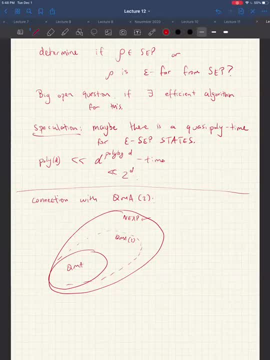 It's not even known to be solvable in exponential time, Right, and which is really in some sense feels kind of embarrassing. So so the answer to this question is: it's not even a problem, right? It could even be NX. 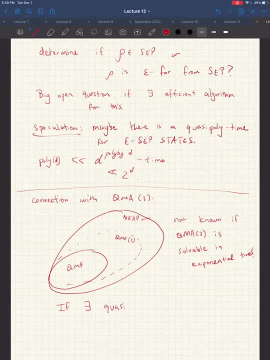 If there exists this quasi-polynomial time algorithm for the epsilon separable states problem. and here it's kind of confusing because I'm saying quasi-polynomial exponential and really in terms of different parameters, but this is quasi-polynomial exponential, so it's a problem. 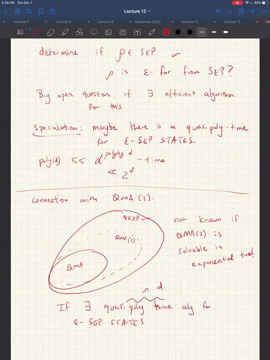 So if there exists this quasi-polynomial time in the dimension D, then this implies that QMA2 would actually be contained in X, And this is because we can reduce the problem to of deciding whether a QMA2 decision problem, you know- is a yes or no instance. 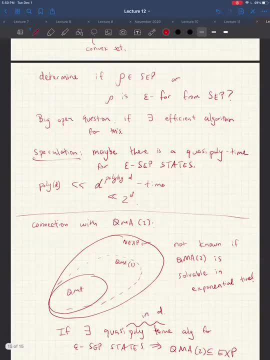 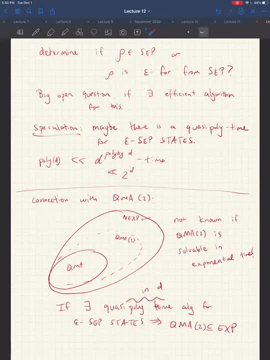 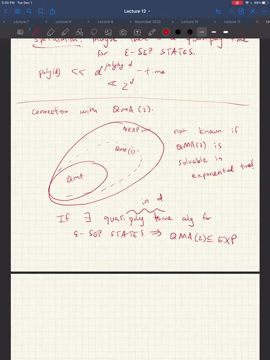 And if we had this quasi-polynomial time algorithm for epsilon separable states, then we can actually do this optimization efficiently in the dimension. But we don't know. So that's kind of why this complexity of QMA2, this complexity of QMA2 really, in some sense. 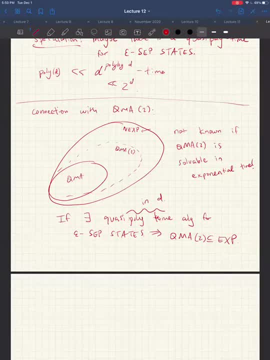 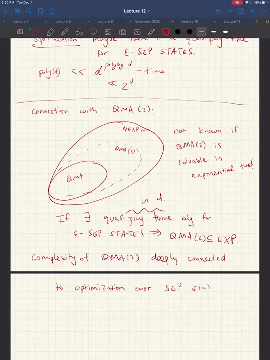 it's like deeply links to trying to understand like, can we actually optimize over these separable states or not? So you know, we before we thought of entangled states as being really complicated. this is telling us sort of a weird you know. 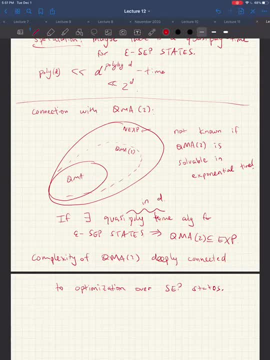 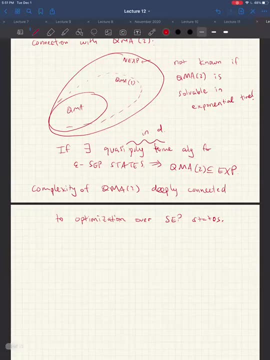 dual version of that, which is that unentangled states can also be surprisingly complicated in some way. The final thing I wanted to mention is that you know, yet another reason why this question is fascinating is because there are connections to these other areas of computer science. 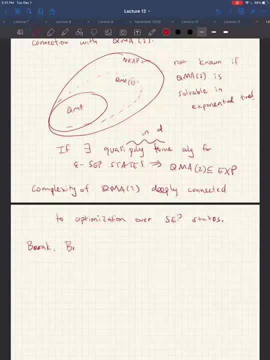 There's a paper by Rock, Brando, Harrow, Kelner, Stor, So a lot of authors. they showed that there's this web of reductions that relate the complexity of the separable states problem to questions in classical complexity theory, namely something called 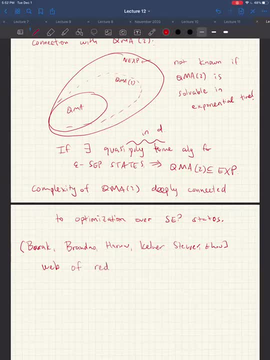 called the unique games conjecture, which is a very big open problem in complexity theory and it has to do with how hard it is to approximate certain optimization problems. So they show that it's NP complete to approximate, assuming unique games. Not quite. I mean-There's some footnote. It comes very close, like if the parameters worked. 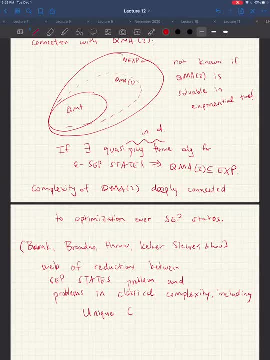 out were just a little different, then it would imply something like that, that it would be like- Assuming the unique games conjecture's hard, then- Yes, Yes, it also be harder, or vice versa, or something. I forget the exact details. 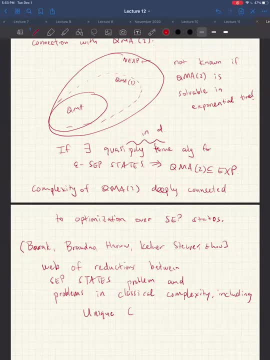 but it could also say something on the fact that if it's hard to solve the separable states problem, then this unique games conjecture would also be true. I forget the exact details, but there's a lot. What is the unique games conjecture? 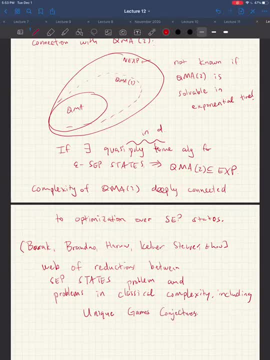 So I guess I don't wanna say out, but it says that a specific type of optimization problem is even approximating it as NP-hard, And it's so influential, it's such a big problem because if this were true then it would imply that so many other natural 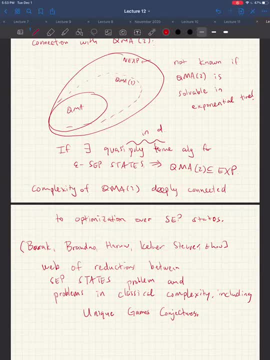 it would tell us exactly how hard it is to approximately solve many other problems. So, like this max cut, this max cut problem that I described earlier, we have a polynomial time approximation out of this problem. There's an algorithm for it that has a certain performance. 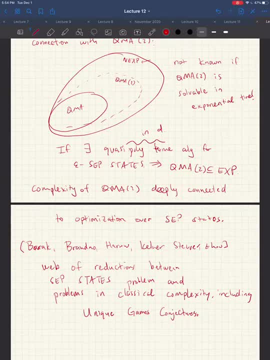 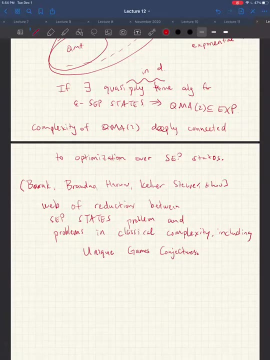 And if the unique games conjecture were true, it would say that this algorithm gives you the optimal approximation. You cannot do any better than that. So, for example, so that's one reason why this unique games conjecture is interesting. Anyways, surprisingly that there is a connection. 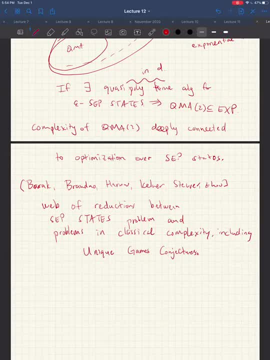 between the separable states and this unique games conjecture, And this long paper that I mentioned really explores the connections between all of these. So, yeah, it really tells us that this QMA2 and this separable states problem and so on are somehow more fundamental. 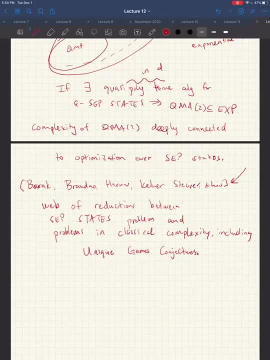 than you might've guessed at first glance. So that's that, that's all I wanted to say about, about QMA2.. So, yeah, and you know for, and finally, yeah, just thank you, very thank you all for attending this class. 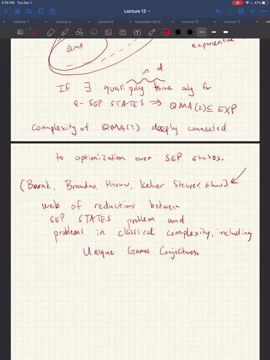 and I hope you found it interesting And, yeah, you know, really looking forward to your course projects. Thank you, Yeah, Thanks for the whole semester. Yeah, Thank you, Thank you, It was a great course. Thank you, Thanks. 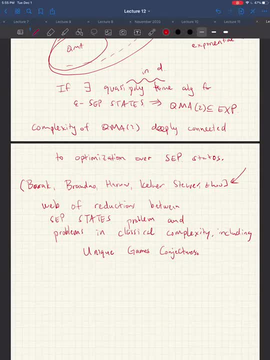 Thanks, Yeah, I really enjoyed the course. Thank you, Yeah, Coming from this quantum information like my, our mind of view- to this new, different view was like pretty amazing, for me at least. Great, I really, I really appreciate the quantum complexity. 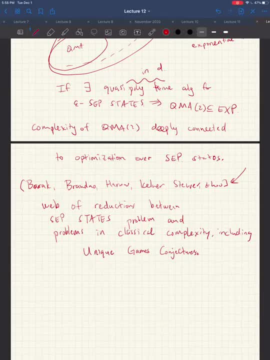 I think I learned a lot because you know I think everyone brought their own perspective and you know. so I definitely learned a lot. Yeah, So you know also, if in the future you know you do more like quantum stuff, I'd be very happy to. 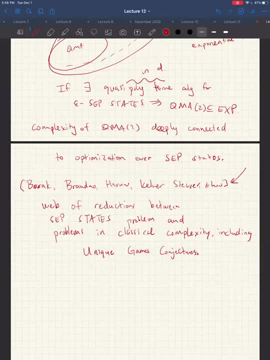 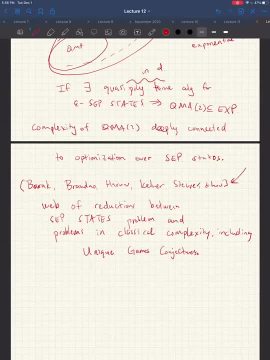 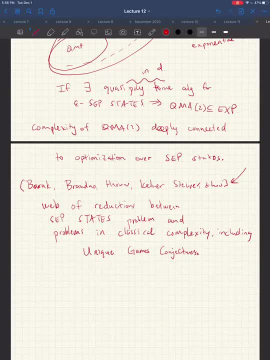 So next semester I'm teaching quantum computing 101.. Yeah, Okay, Sweet, I think. the introductory courses is, I think, harder to teach. Yeah, probably more important though. yeah, all righty. so, um, uh, have a safe, uh, you know, rest of december and, you know, take care of yourselves. 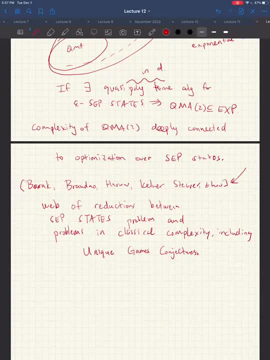 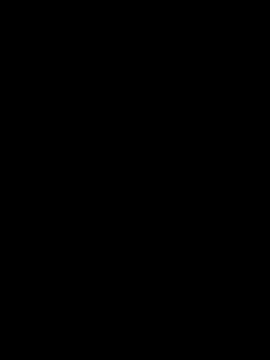 all right, bye everyone. okay, thank you, thank you again. yeah, thanks, bye. good night you.